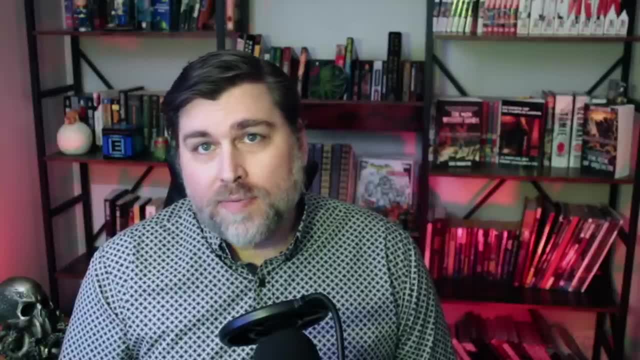 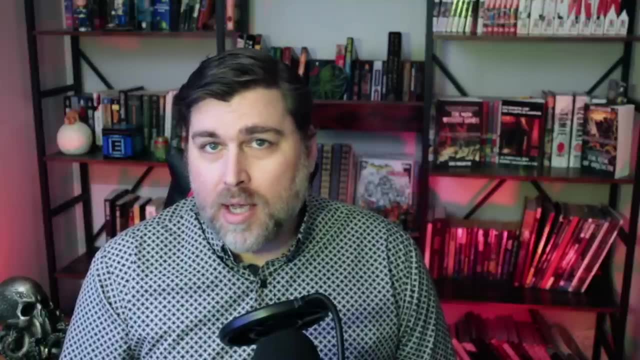 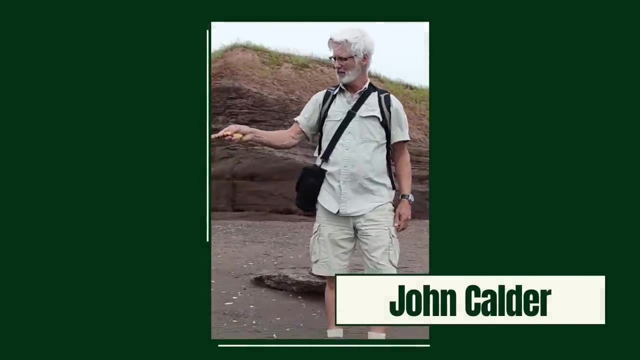 on the western coast of Nova Scotia, Canada. Three hundred and fifteen million years ago it was an equatorial forest. The cliffs below Joggins are a UNESCO World Heritage site. Dr John Calder, who was instrumental in securing that recognition, calls them the storybook of the Coal Age. It is a book to. 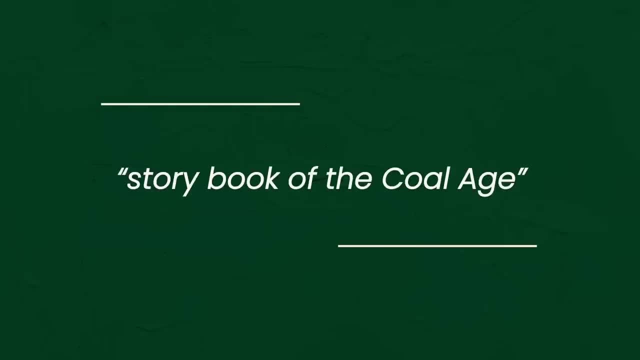 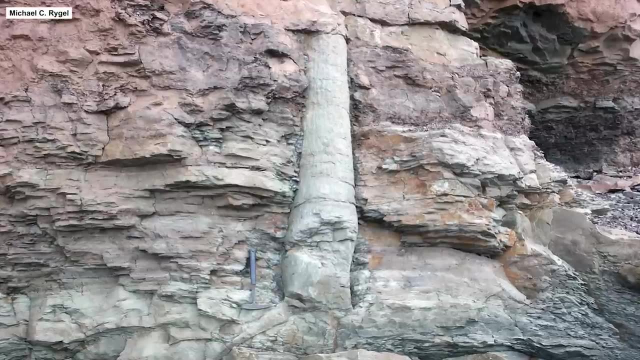 be read in wonder, but not lightly To Calder. the cliffs hold great lessons for us about our shared past and our future together on this changing Earth. Here and there, embedded high in the face of the cliffs, are what appear to be Grecian columns. 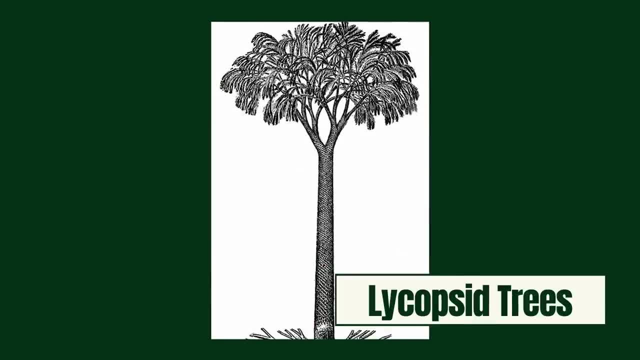 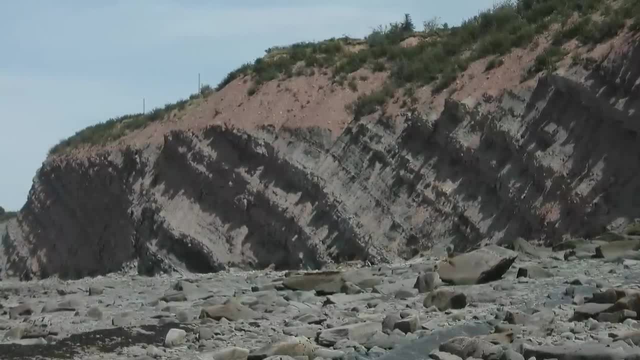 The columns are the trunks of fossilized, lycopsid trees, kings of the Coal Age forests. Within the layers of rock, sixty ancient forests are still standing. Their trees are upright and hollow, their stone roots reaching deeper than in life. Small creatures are entombed. 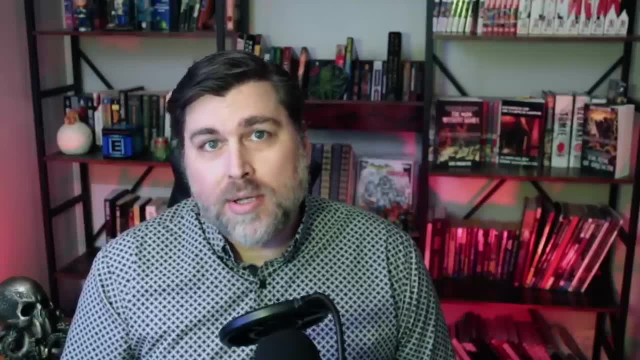 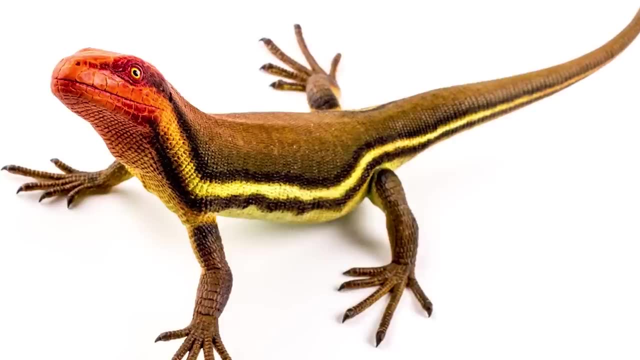 inside the trees some of the earliest land-dwelling vertebrates. One is Helanomus yelli, the first reptile in the fossil record. After three hundred and fifteen million years in darkness, erosion is pulling them all back into the light. 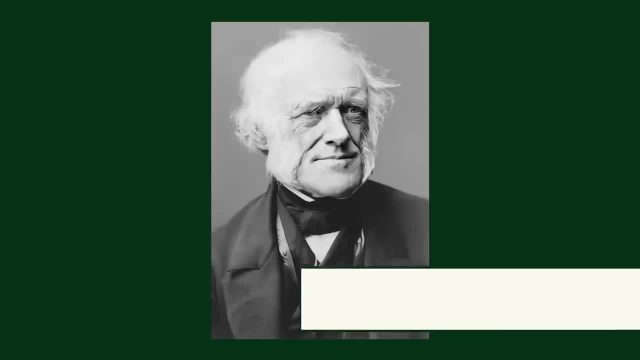 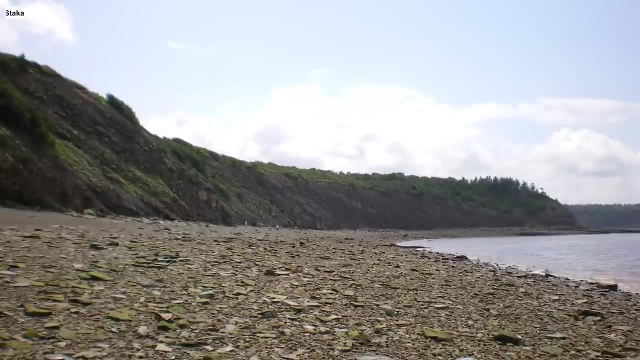 The first hollow tree creatures were discovered in 1852 by the famous Scottish geologist Sir Charles Lyell and his colleague Canadian paleontologist Sir William Dawson. But you might equally say that the creatures discovered them by crashing down onto the beach at the 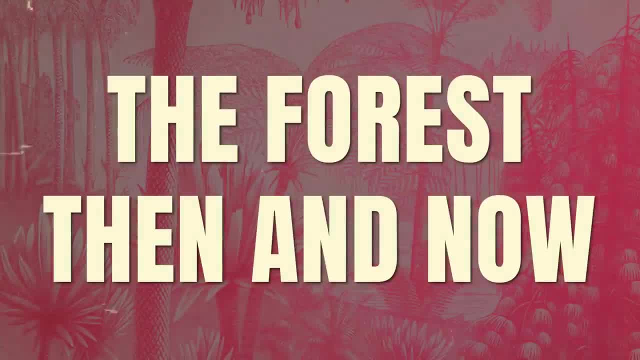 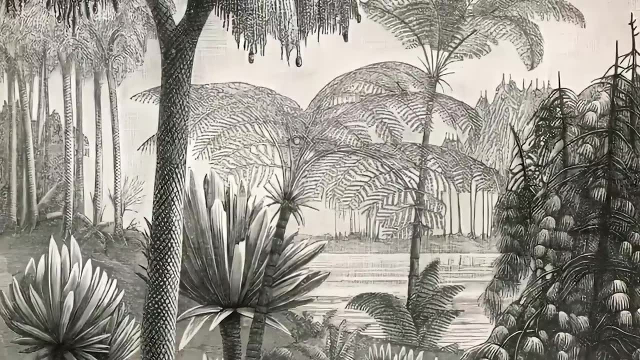 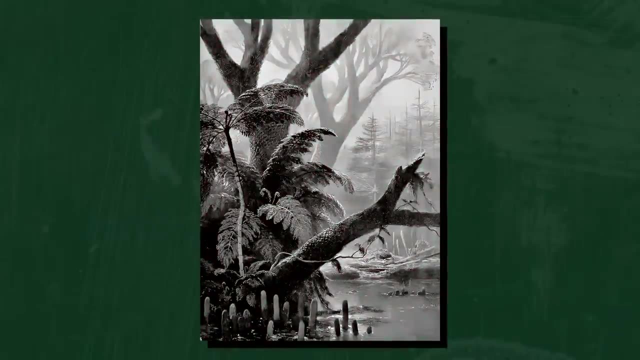 right time. In the storybook of the Coal Age, the Swamp Forest is a temple to itself. The lycopsid columns of the temple stand a meter thick and thirty high, Decorated in the shape of an elaborate and delicate geometrics, some of them branch symmetrically at their crowns. 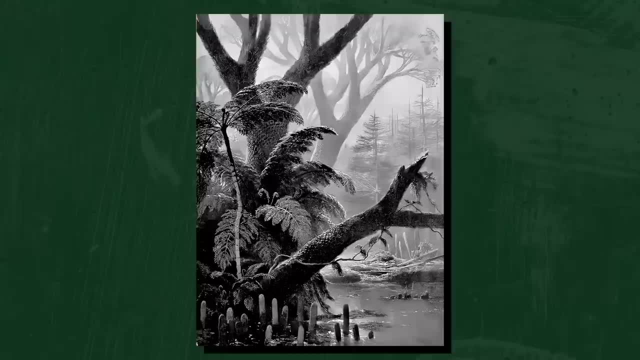 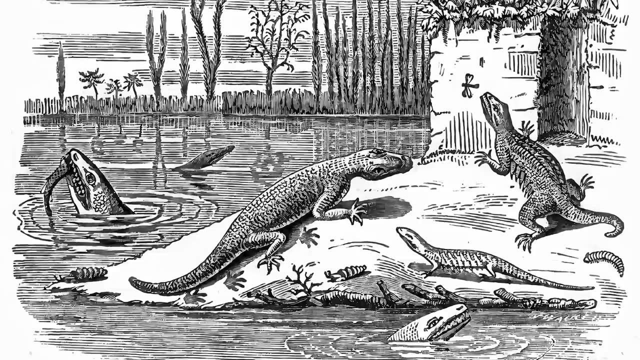 making vaults. The roof of the temple is a distant canopy of needles and cones shaping strange windows out of the sky. Many fossil forests already sleep in the rock beneath this one, but Helanomus knows nothing of that. Helanomus is lithe, fast and sharp-toothed. 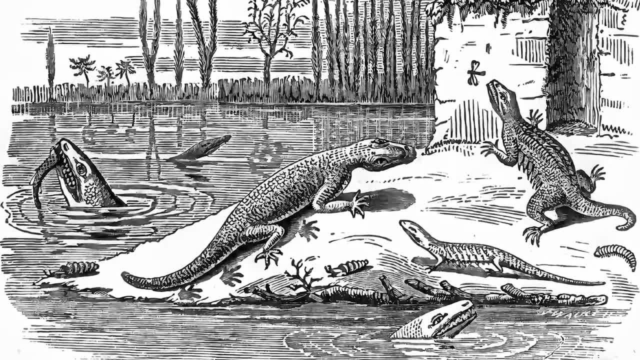 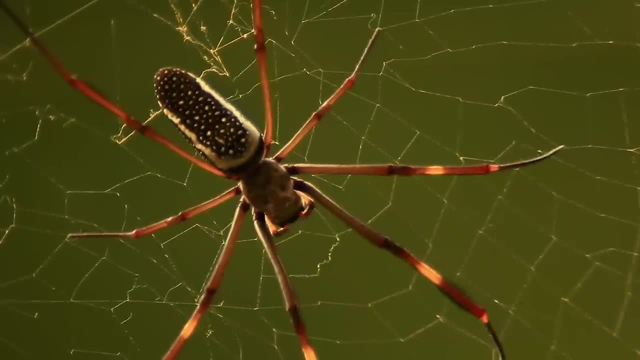 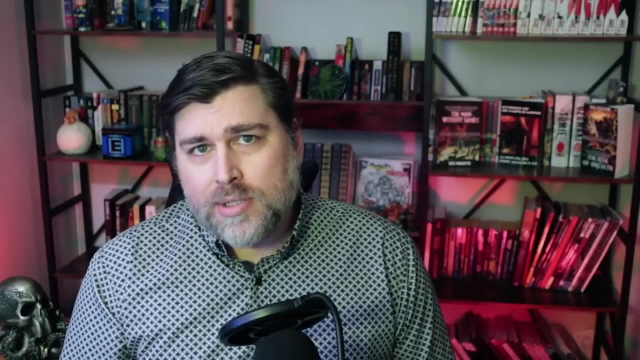 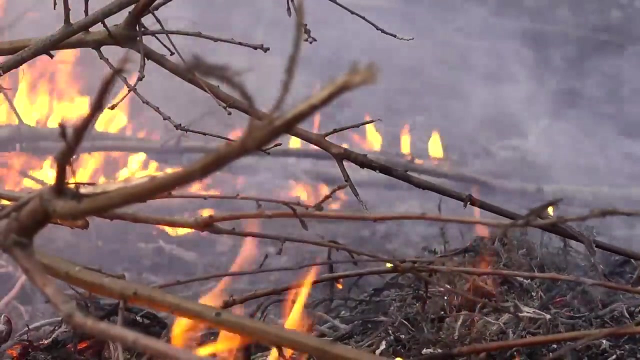 million years. There are no birds or no mammals. There are palm-size spiders, giant dragonflies and two-meter-long millipedes. Invertebrates grow monstrous here in the oxygen-heavy air and lightning strikes catch fire instantly. When the fires roll through, Helanomus knows where to go. Its den is an inner sanctum of. 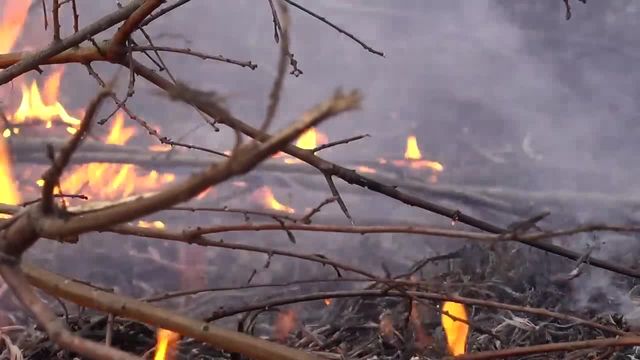 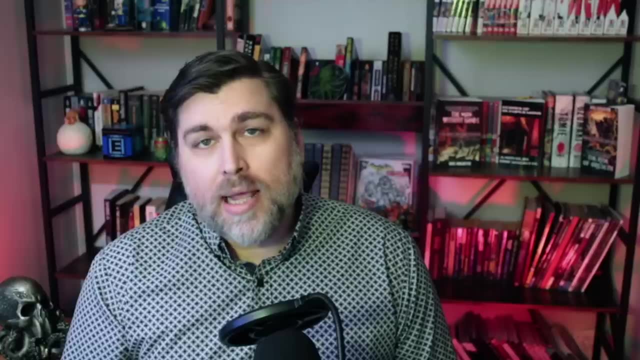 the Forest Temple, a hollow like Hopsid, the door carved by fire. The flames reach in again, the winds impl apparat them to beat down the trees, to cleanse their IMG, Then Helanomus. but when the fire passes, Helanimus is safe. One day, days or years from now, Helanimus will not. 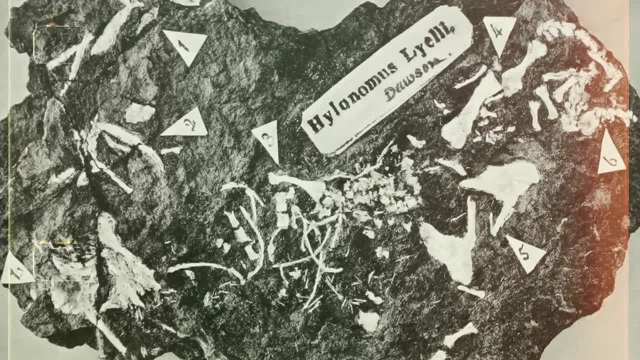 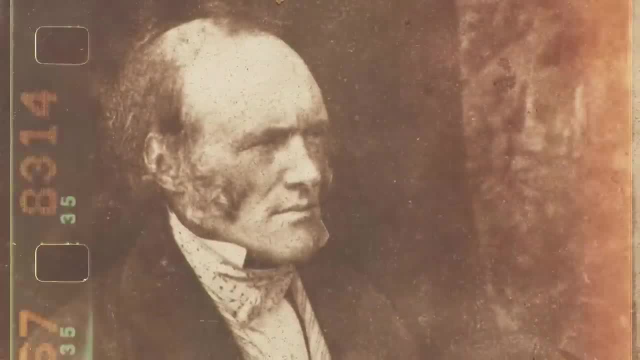 leave its den, The hollow tree will fill with earth and turn to stone, and they will be interred together in the great mausoleum beneath the forest temple, 315 million years later. Sir Charles Lyle will go looking for them. He won't know. he is looking for Helanimus, He's looking for the 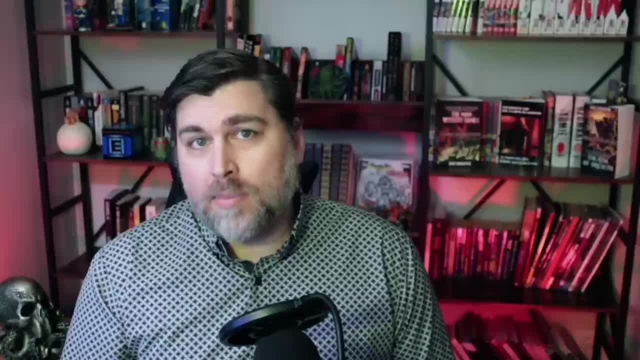 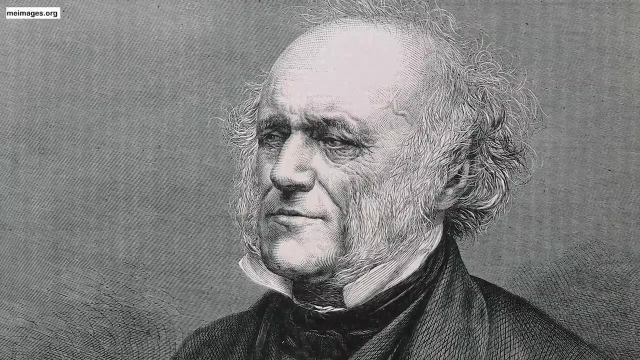 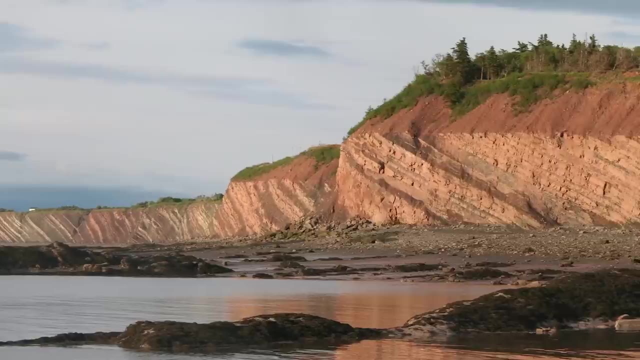 answer to Cole. He's looking to prove himself right about deep time and to prove Charles Darwin wrong about evolution. When Lyle's boat approaches the cliffs of Chagogan in 1842, he will see the great book opening before him. The cliffs appear as a 15-kilometer-long stack. 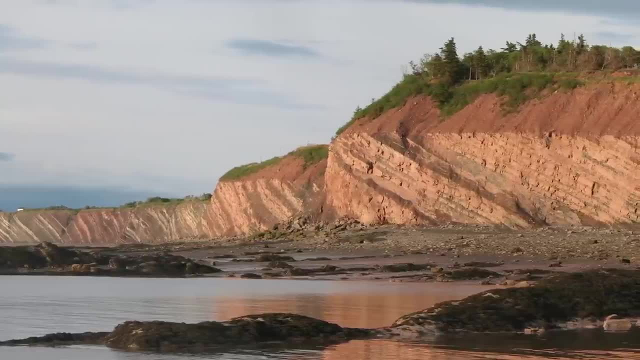 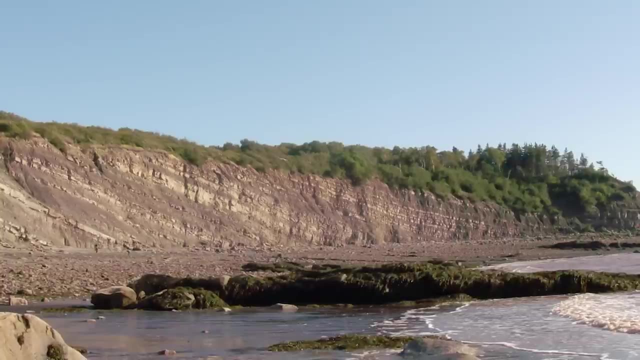 of pages leaning 20 degrees against the side of a shelf. Every page is a layer of sedimentary rock, vibrant and distinct Sandstone, siltstone, mudstone, limestone and coal. At the base of the cliffs, the sandstone layers extend outward into the bay. 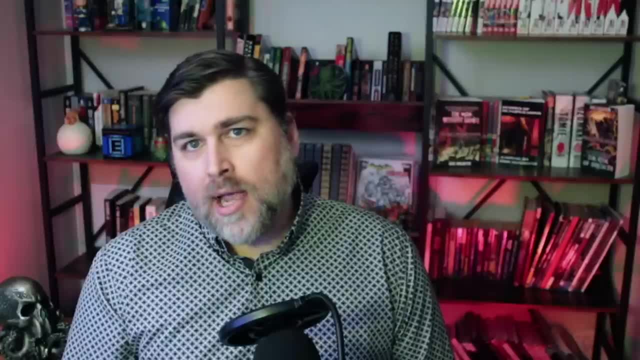 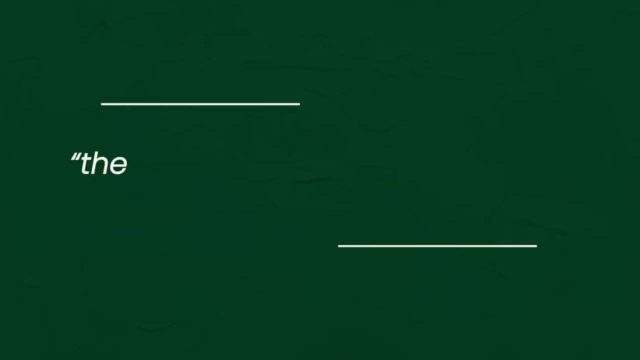 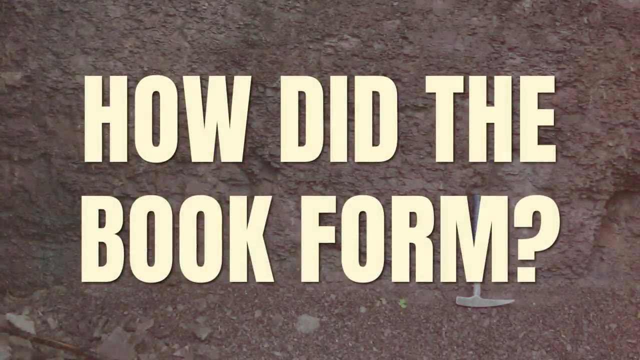 Forming a series of massive intertidal reefs At low tide. the book of cliffs can be seen with its pages open, inviting itself to be read In a letter to his sister. Lyle will call it the most wonderful phenomenon that I have seen. Before it was an open book. Chagogan's was a. 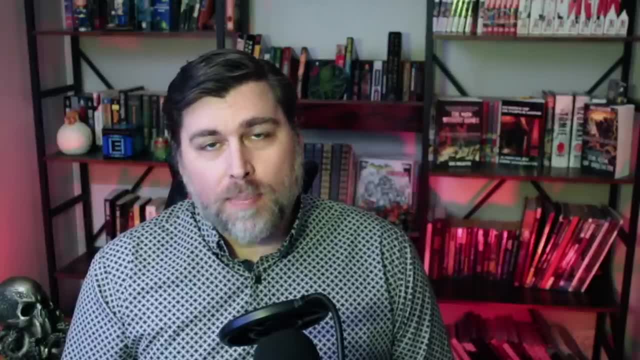 buried ream of pages, a thick stack of sedimentary rock beds. The ream became a book at the end of the last ice age, around 13,000 years ago, When a glass of ice was poured into the ream. the 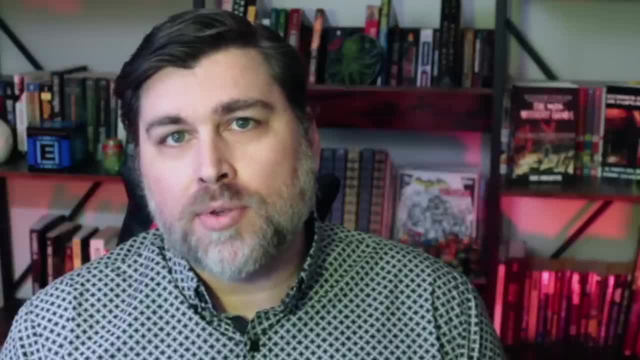 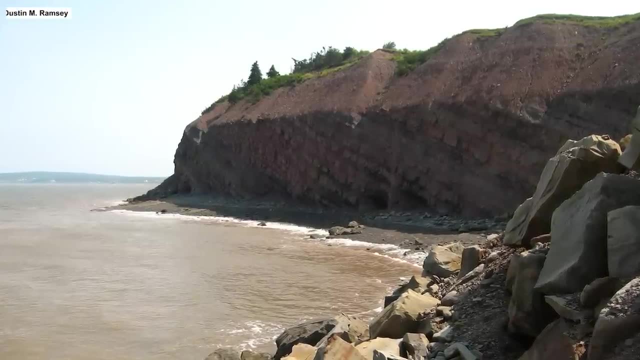 glacier retreated from the former shore, The long compressed earth sprang upwards and the cliffs rose. Since the exposed layers tilt to the south. when you walk north along the cliffs, you are walking backward in time At Ragged Reef, the southern point of the World Heritage Site, the 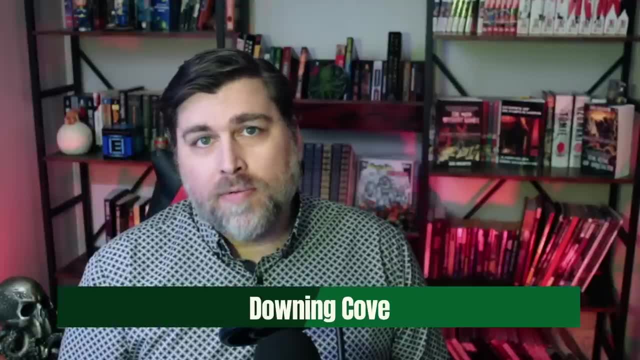 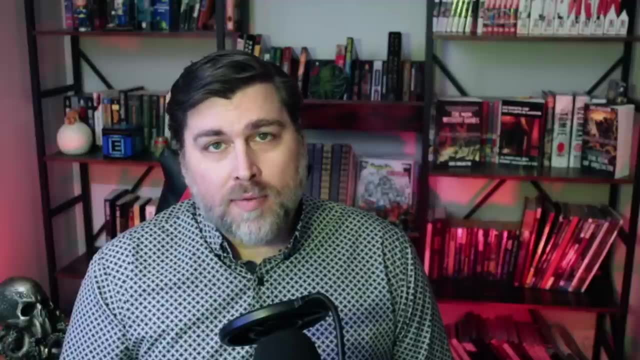 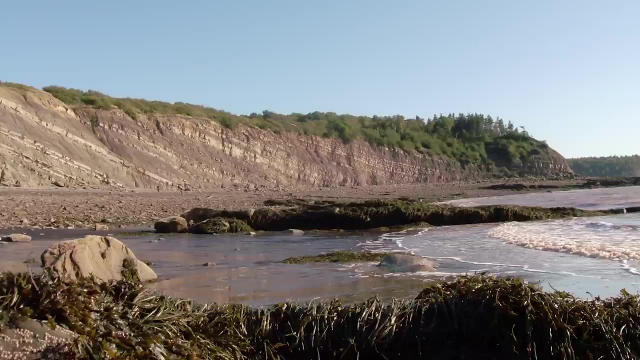 layers are 310 million years old. At Downing Cove, the northern point, they are 325 million years old. In 15 kilometers of beach you walk 15 million years. Once this slice of time was exposed, the tides took a cudgel to it: Tides along the Chagogan's. 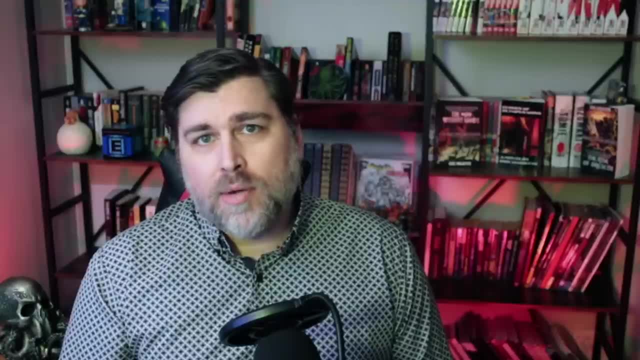 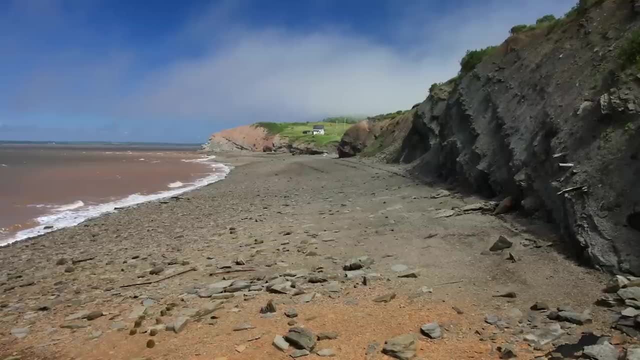 coast are the most extreme in the world. Every day, the shoreline rises and falls 16 meters as 100 billion tons of water move in and out of the Bay of Fundy. Under this barrage, the cliffs are continuously reshaped. Large sections fall regularly along fault lines. 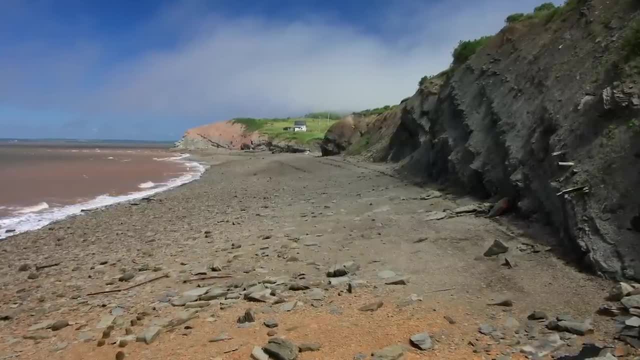 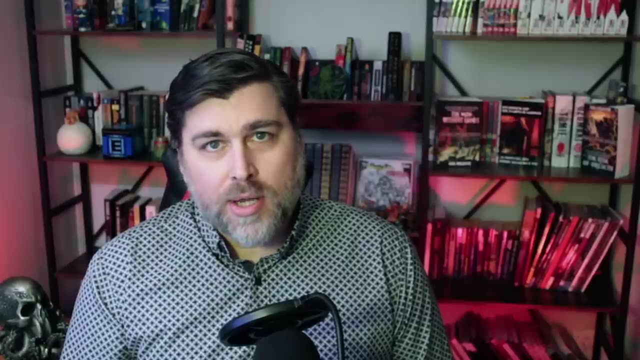 chiseled by the harsh frosts and thaws of Nova Scotian winters, New trees are revealed before crashing down onto shore. Old mines are found on the shore and new trees are found on the shore. The mine workings are exposed tunnels into another dark past. The water takes away newly. 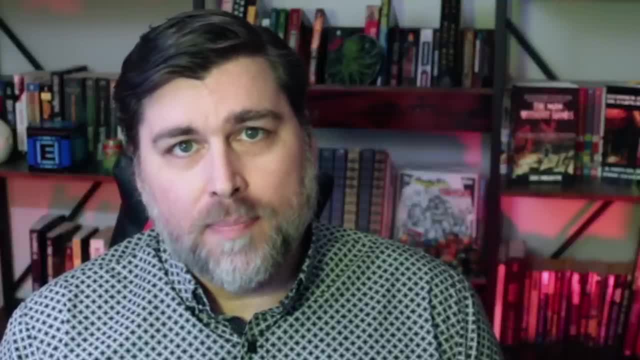 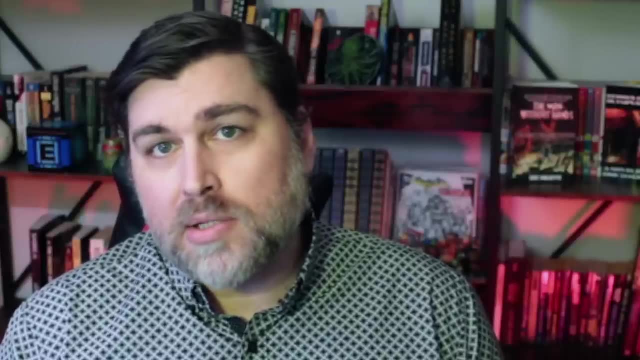 fallen rocks and fossils, burying them or destroying them. As it buries, it unburies. Every day. there is the possibility of a new breakthrough discovery. Every day, something is lost, forever, never to be known. The past is frozen, unchanging But our path through. 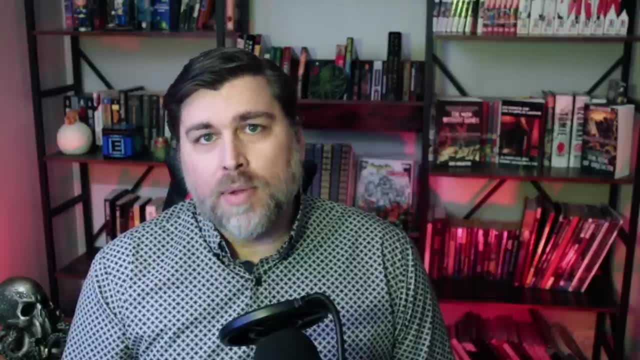 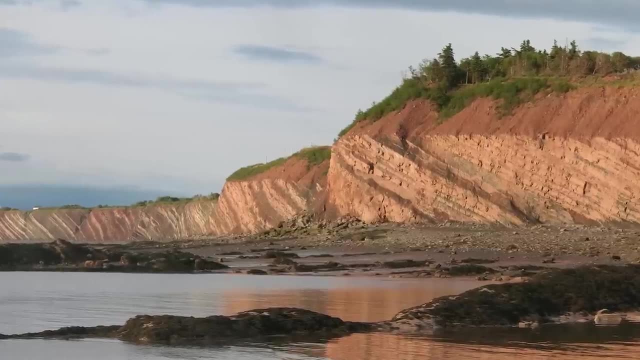 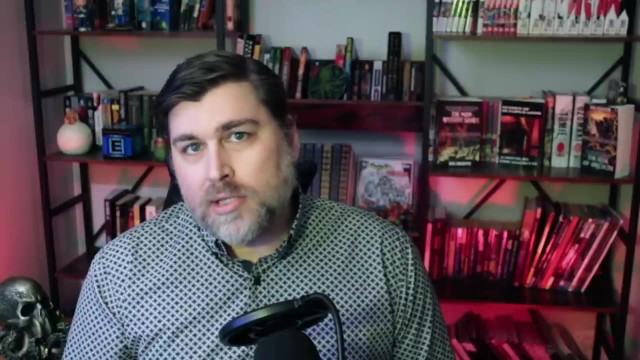 the past is ever-changing and looks different all the time. At the north end of the beach, the cliffs are tan and sandy. To the south, they are jagged and gray shot with coal. This boundary marks a worldwide change in climate, one that splits our category. 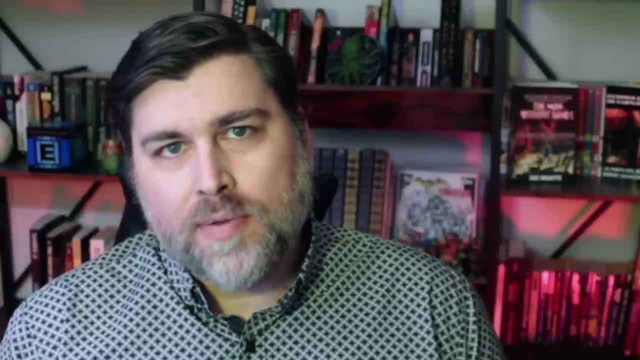 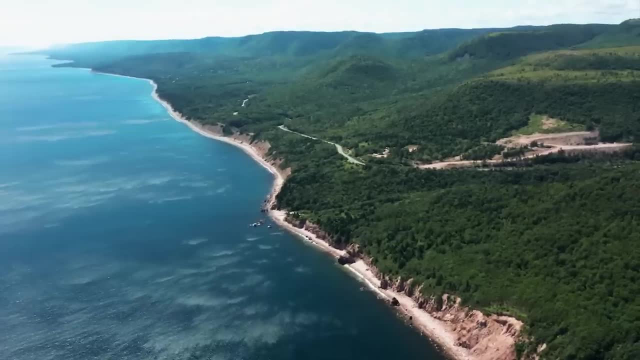 of the Carboniferous Age in two. During the early Carboniferous, the future shores of Africa and North America crashed against each other. They razed the Appalachian Mountains and the highlands of Nova Scotia and Scotland. Huge rivers flowed down from the new mountains, washing in sand and 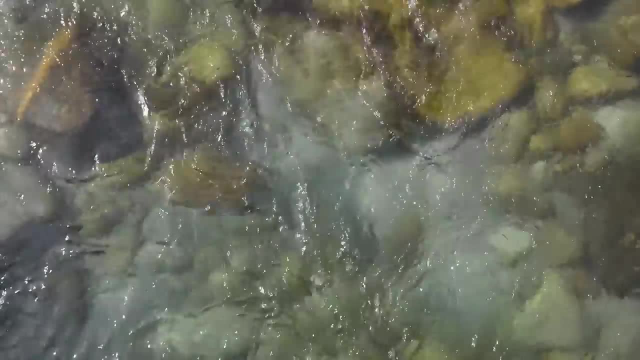 far-flung fossils creating the sandstone lake At the north end of the beach. the cliffs are unchanging. There are still layers at the older end of the beach. Plant fossils from the early Carboniferous lack growth rings suggesting indistinct seasons. 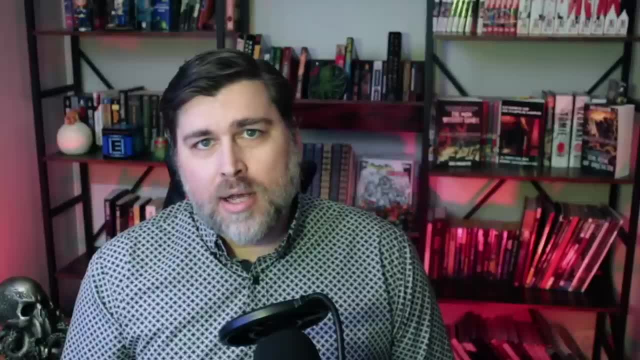 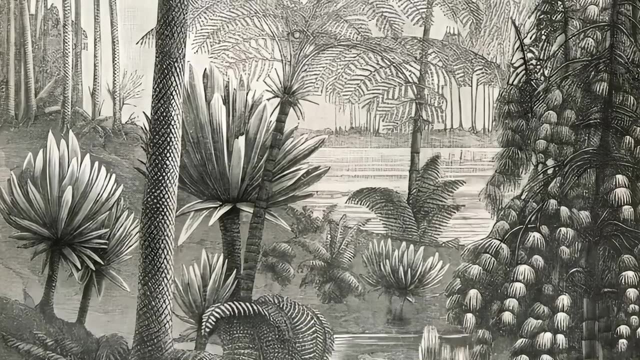 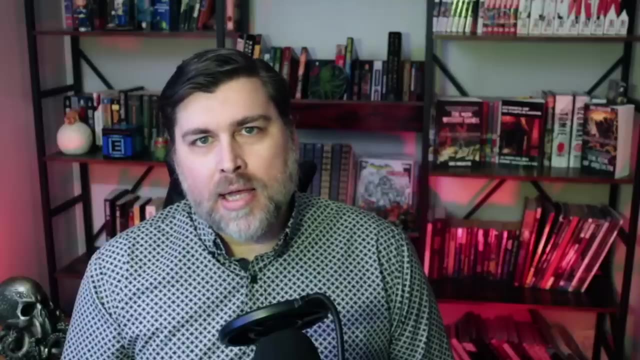 The climate was hot, humid and globally consistent. The shifting continents created more land, which was alternately flooded and dry. These were the perfect conditions for lycopsoid swamp forests to spread across Europe and North America, and the perfect conditions to make coal. The plants took carbon dioxide out of the air, using it to create their substance. 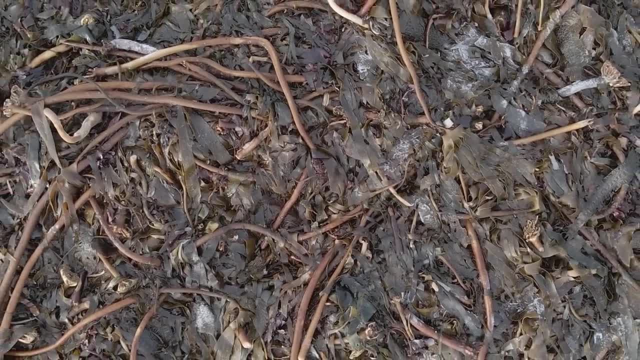 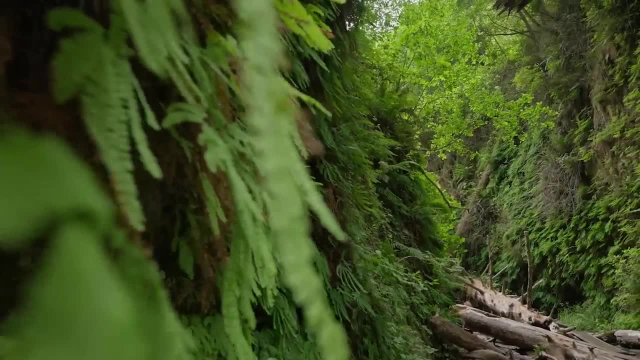 Dead plant matter built up as peat, Still storing carbon, and didn't fully decay. Compress the peat for a few millennia and you have coal beds. As plants take carbon dioxide out of the atmosphere, they put oxygen into it. 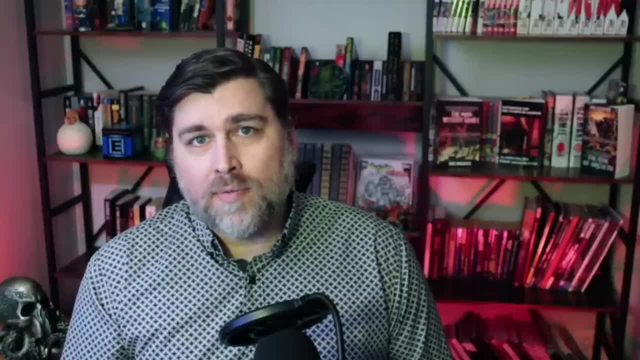 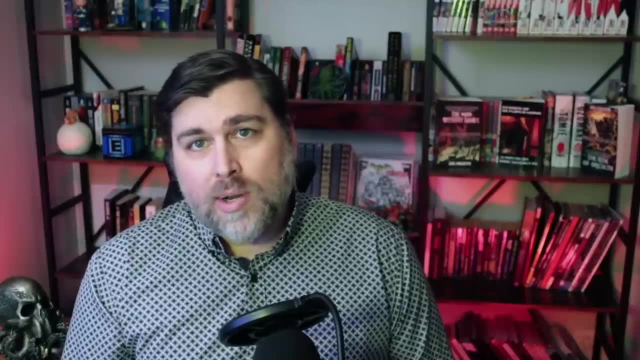 In the late, Carboniferous oxygen concentration rose higher than ever, 50% higher than today. A high-oxygen, low-carbon dioxide atmosphere had the effect of cooling the earth, the opposite of the greenhouse effect we see now. Temperatures became milder and the South Pole 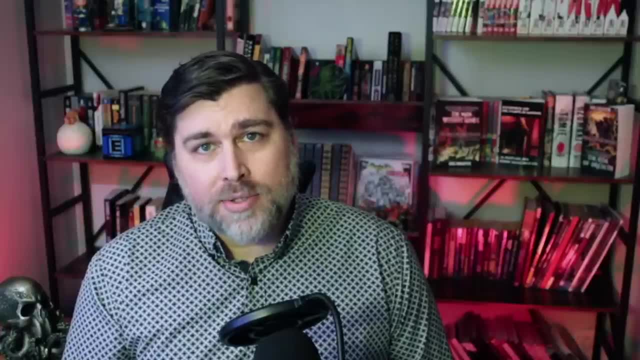 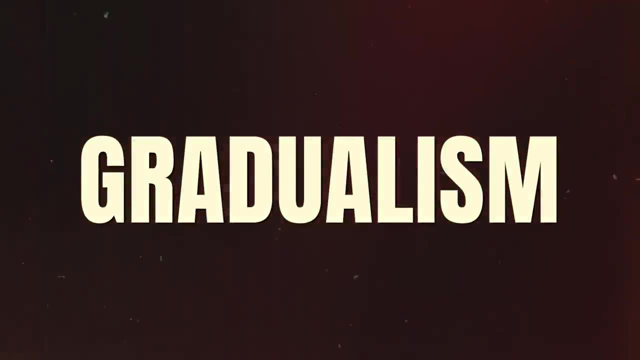 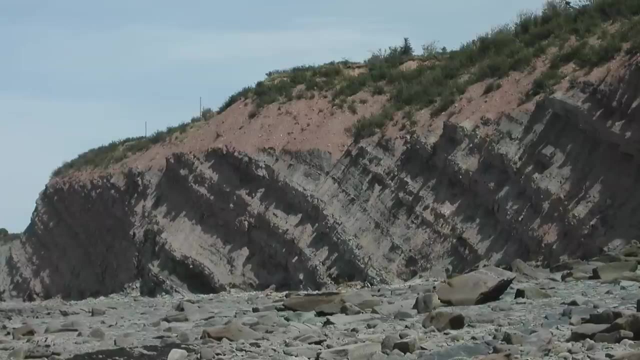 froze At Joggins. the topography changed from drylands to wetlands and the swamp forest began to grow. The book of Joggins shows, layer by layer and year by year, how the change happened. As you follow the cliffs south, thin beds of coal start to appear. Over time they get thicker. 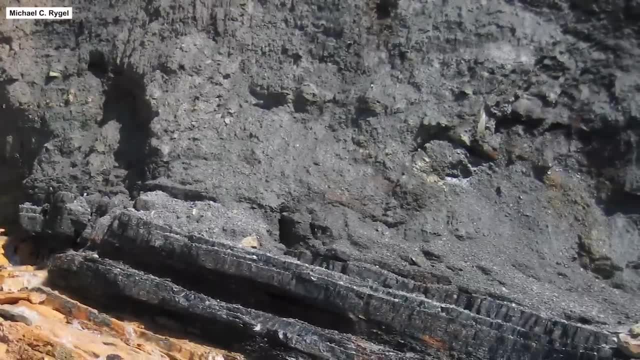 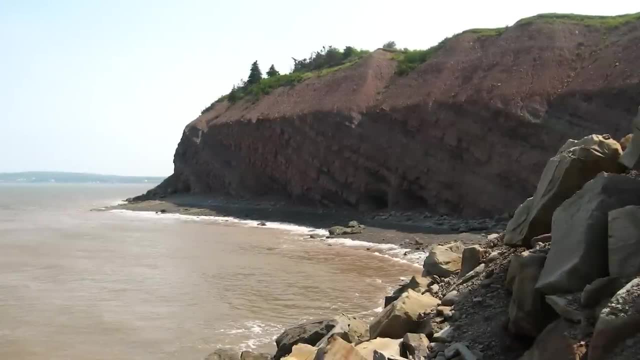 and thicker, eventually thick enough to be mined. Over 67 beds of coal are exposed at Joggins, and sandwiched therein are the 60 forests. The picture of gradual change over time is exactly what Lyle was hoping to find at Joggins. 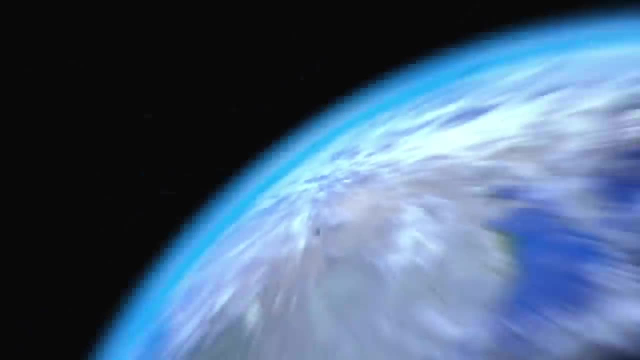 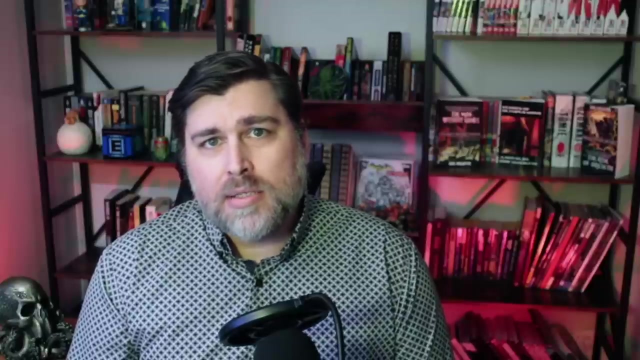 Lyle was the world's leading proponent of the theory of gradualism, which held that Earth's timeline was vast and the planet had changed extremely slowly. The competing theory, catastrophism, said the Earth had only been altered over time by rare, momentous events. 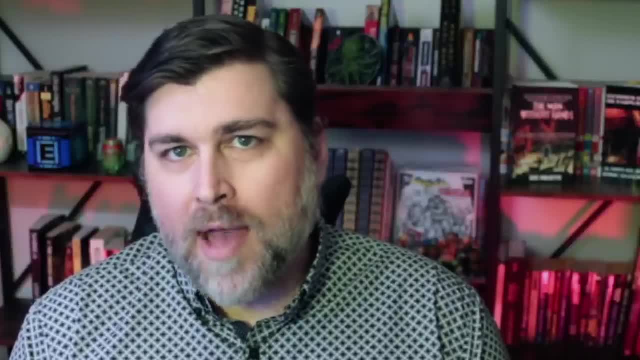 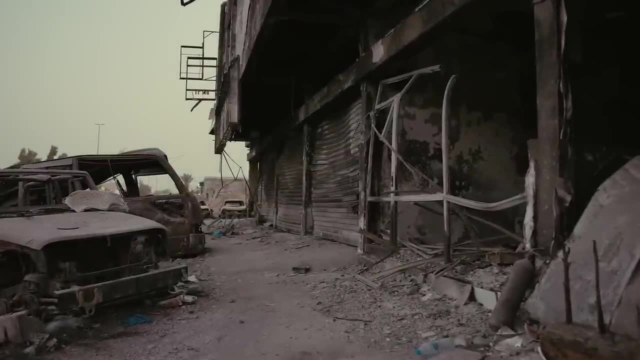 The story of gradualism versus catastrophism starts half a century earlier, when a worldview-breaking idea was added to our understanding of species: the idea of extinction. In 1787, giant mystery bones were discovered in America and fancifully 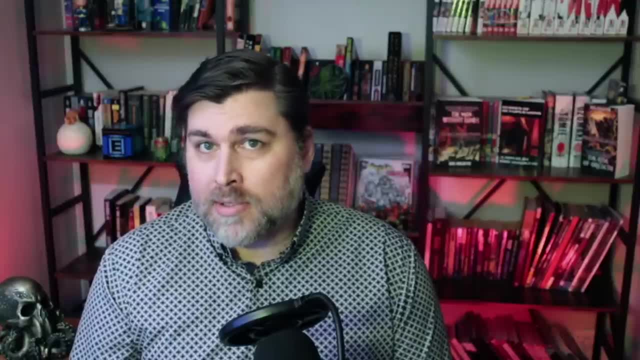 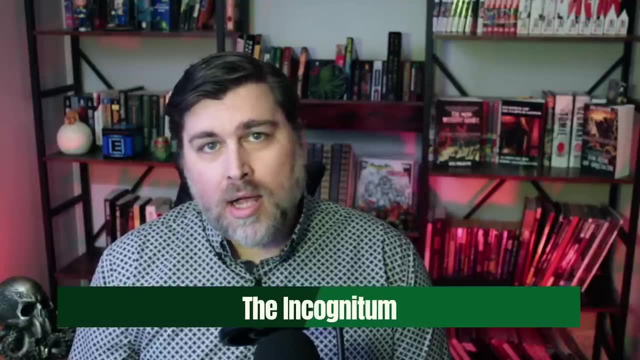 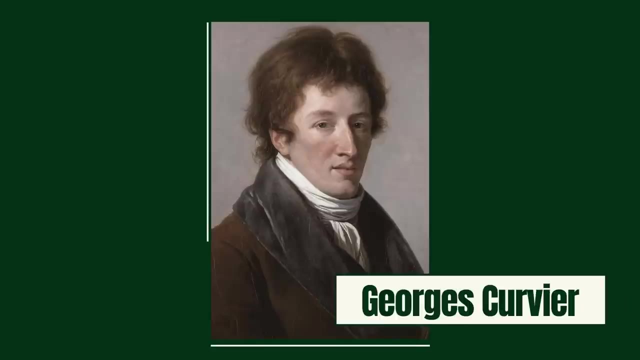 interpreted into an elephant-like creature six times its size. It had the claws of a giant sloth, the grace of a tiger and tusks on top of its head. It was called Incognitum. No one could agree what it looked like, but it definitely wasn't around anymore In 1796, hotshot paleontologist Georges 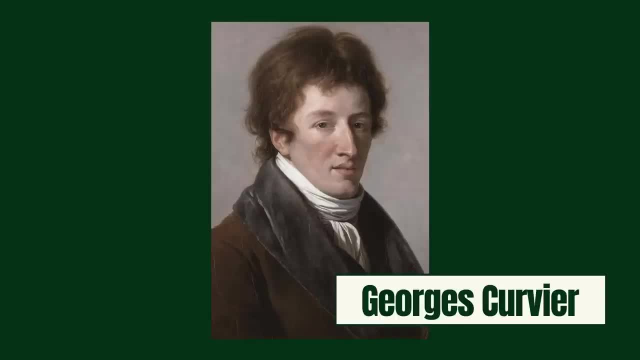 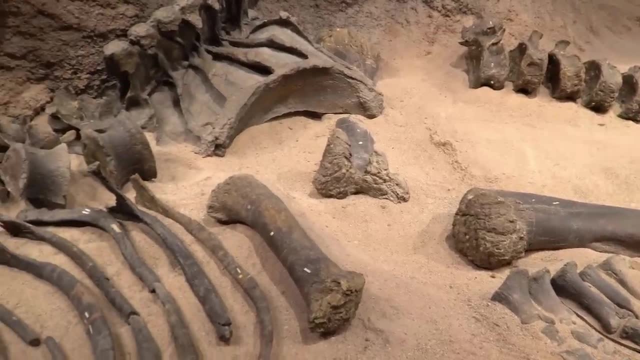 Curvier wrote a paper describing for the first time a theory of extinctions. He put the blame on forgotten global catastrophes. Extinctions sat badly with the dominant Christian worldview of the time. Life was supposed to be here for a reason. Why had the Incognitum been made only to be? 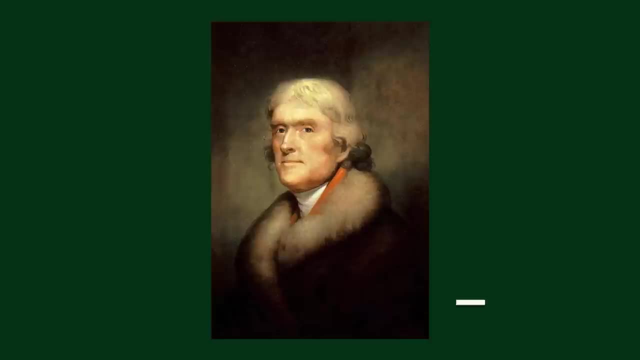 destroyed. It seemed too casual, too purposeless. When the American President Jefferson sent an expedition to explore America's interior, he was hoping his scientists would find herds of macedons somewhere and prove extinction wrong Over the next 50 years. a schism emerged in 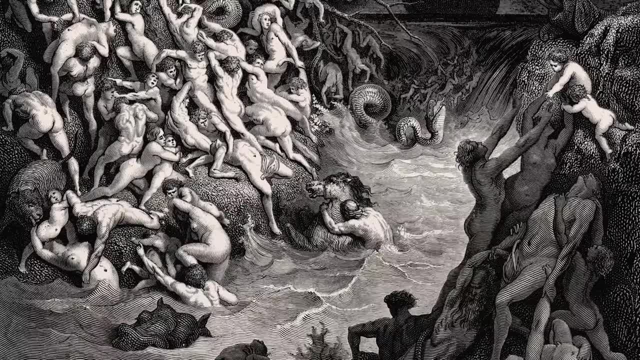 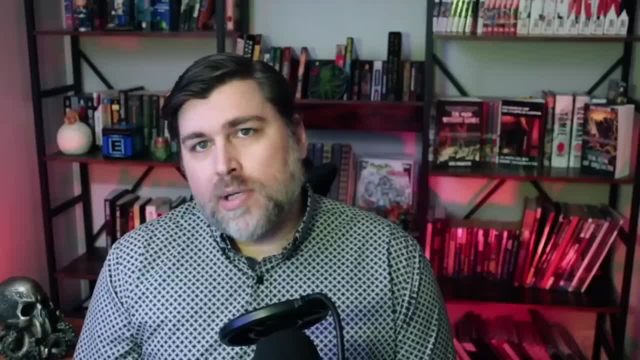 paleontology. Catastrophists versus Gradualists. Catastrophists believed events like the Biblical Flood had ended species, leveled mountains and changed the world. They believed that the Earth changed by large steps. Gradualists held that the Earth changed very slowly. 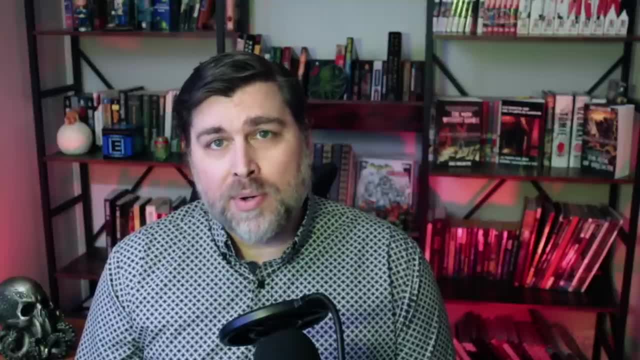 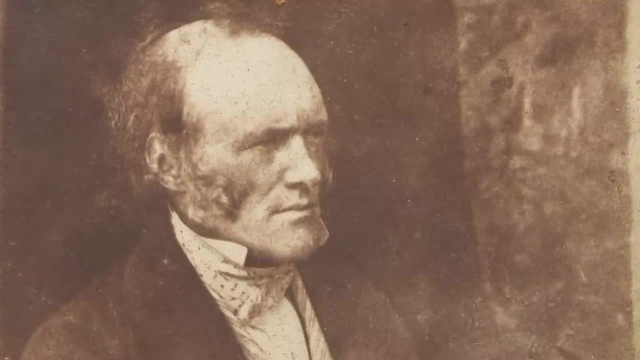 and that being the case that it must have happened over a vast period of time. Lyell became Gradualism's biggest champion. He believed the present is key to the past, that whatever happened back then is still happening now. He looked for evidence that. 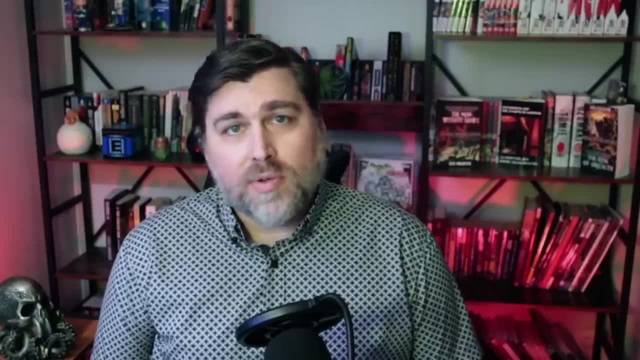 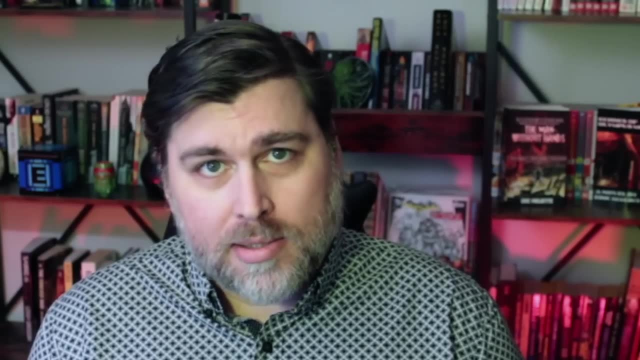 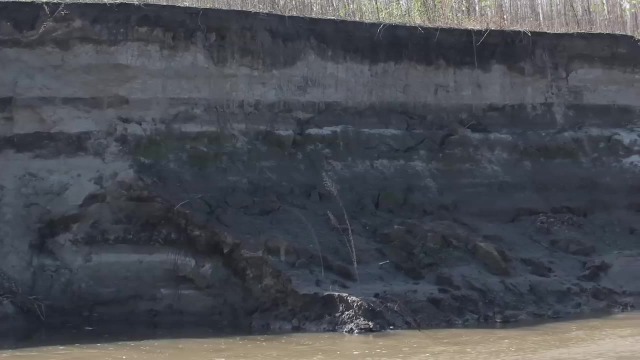 the Earth was shaped and reshaped by the same familiar rivers and tides, the same forces of erosion and decay that we see all around us. He found that evidence at Joggins. A layer of sediment is a layer of tiny particles. The particles were moved into place by flowing. 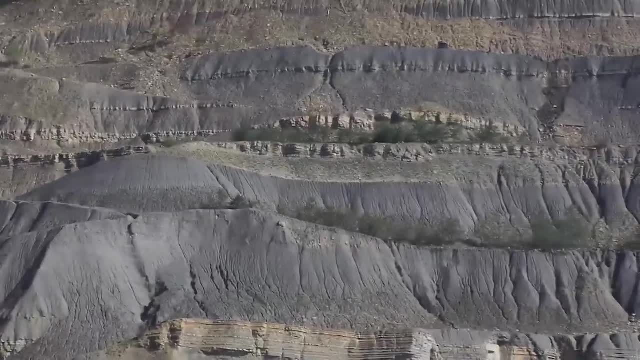 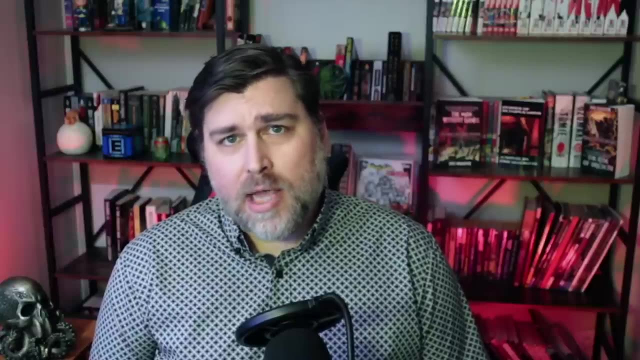 water. then they settled and solidified. Therefore, each layer records an event that moved sediment into place. The layers have different features depending on the size and type of particles that form them and the nature of the moving water. By looking at the features, 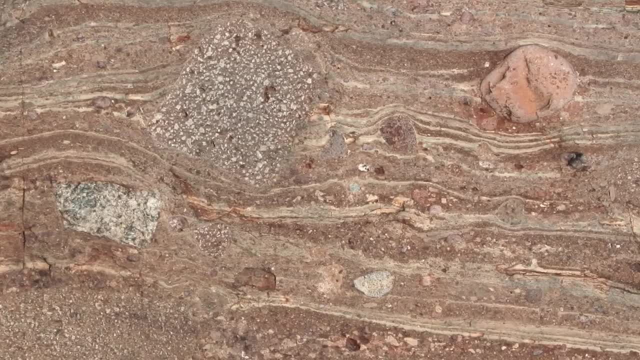 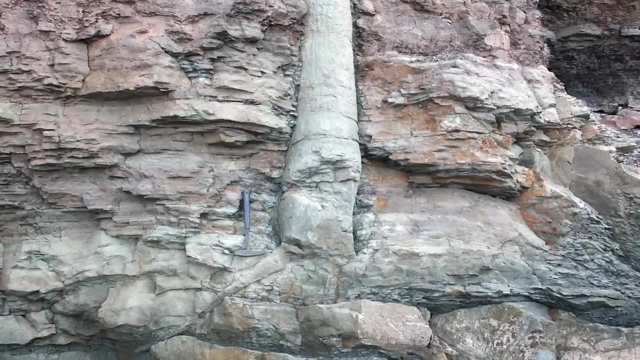 of a layer, we can make a guess about the event that caused it and what span of time it represents. Look at the layers that contain buried trees. How did the trees get buried? How long did it take? A buried trunk is encased in many thin alternating layers of sandstone and mudstone. 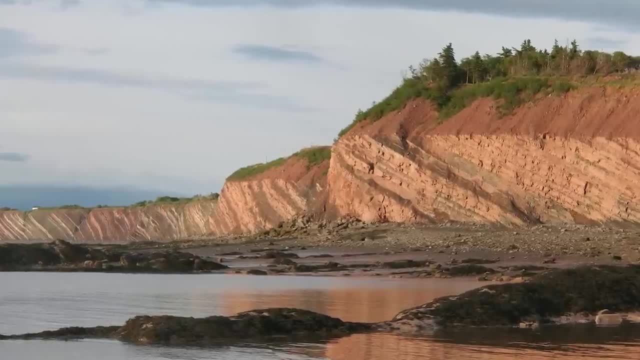 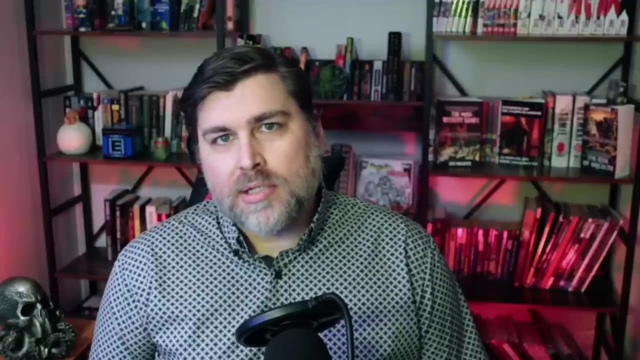 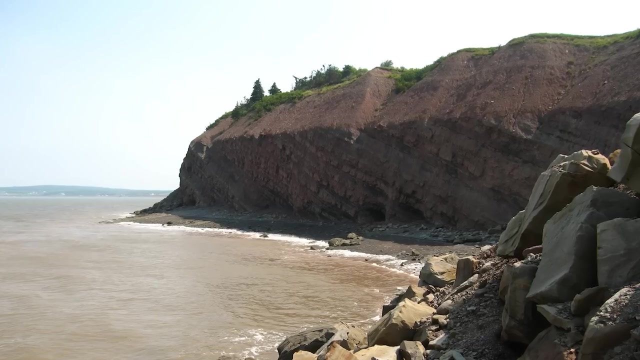 The sandstone layers have a sharply defined base and a top that graduates into the next mudstone layer. The pattern is what we see in climates with seasonal flooding. Floodwaters move sand into place and the large particles settle quickly. Smaller mud particles settle more gradually on top of the sand. We don't know how frequently the 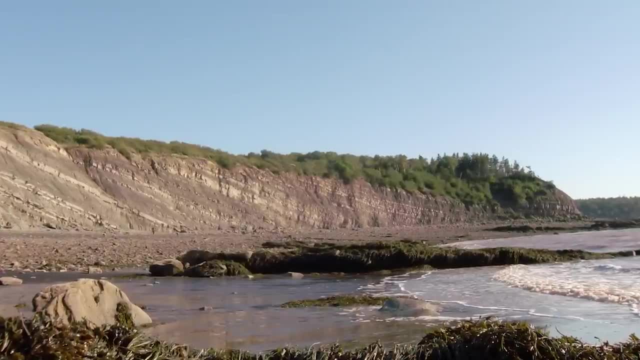 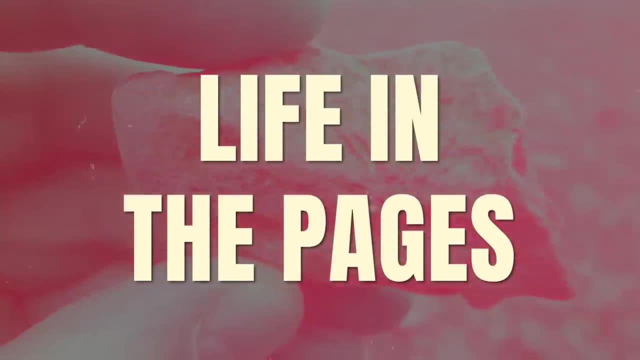 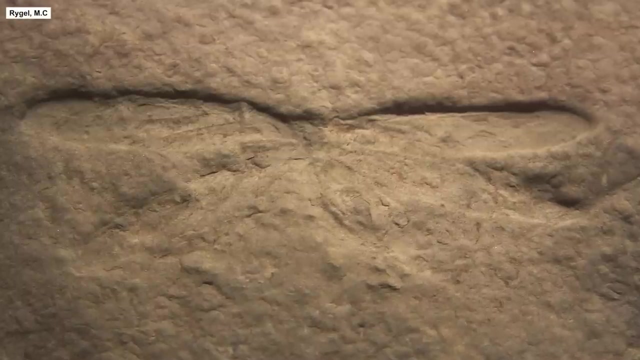 mud particles move, but we can speculate that a four-meter trunk was buried in less than 40 years. When separated, the layers of sediment can be read. The fossilized footprints and trails of coal-age creatures show us how they lived. A heavy amphibian twisted its feet as it walked. 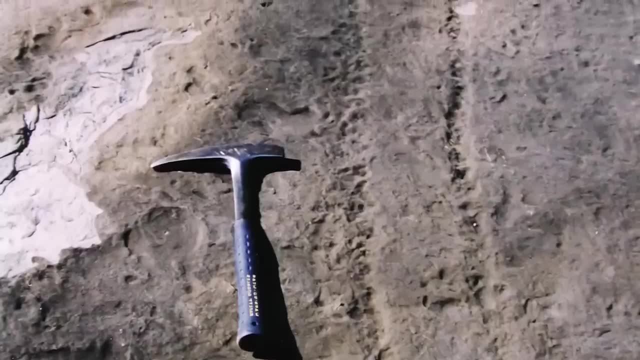 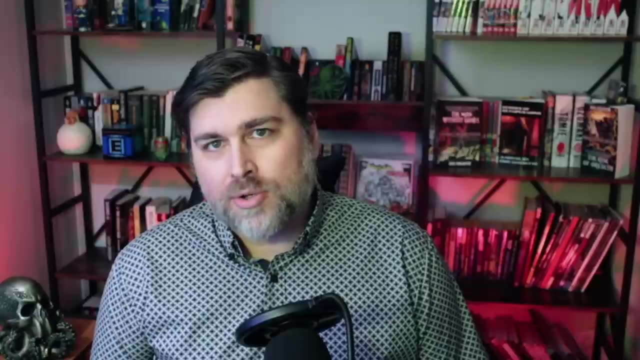 pulling them out of the sticky swamp mud. A smaller tetrapod dug its claws in Something huge and many-legged, left trails like truck tires. We can compare the fossil tracks to the tracks of modern animals to imagine how they moved and behaved. Impressions of strangely patterned bark. 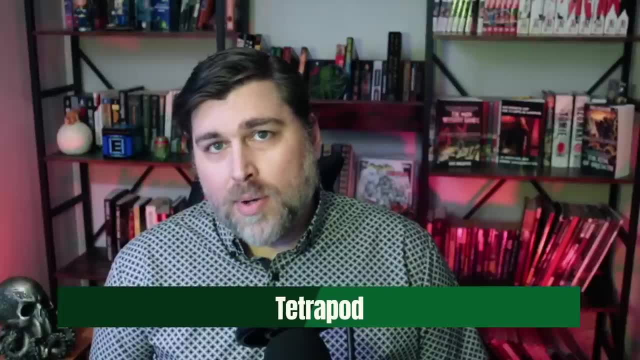 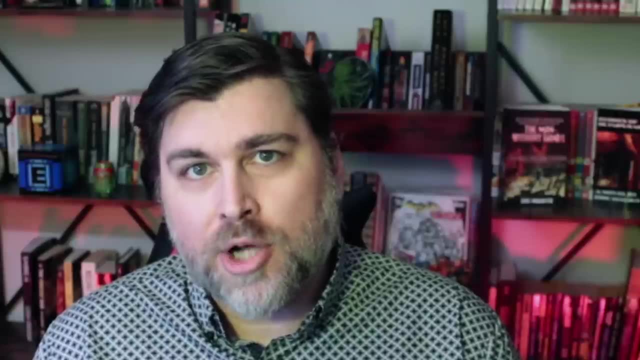 and intricate fern leaves are abundant. Fossil tetrapod bones are relatively rare. A tetrapod is a land-dwelling amphibian or reptile. Nineteen species have been discovered at Joggins, from the size of a salamander to the size of an iguana. 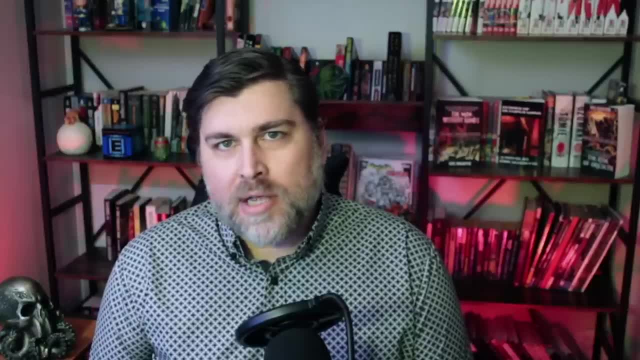 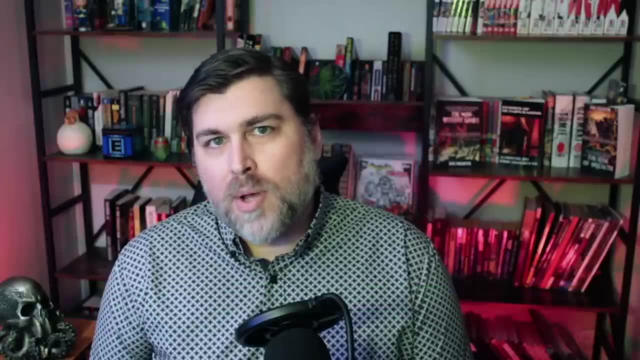 315 million years after they lived. a few of these tetrapods became famous. The hollow-tree creatures, as they were called, are the iconic discovery at Joggins: Fossil bones interred inside the fossil lycopsoid trees. Dawson collected hollow-tree creatures at 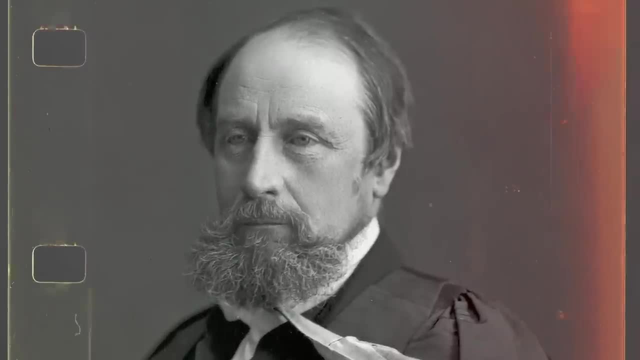 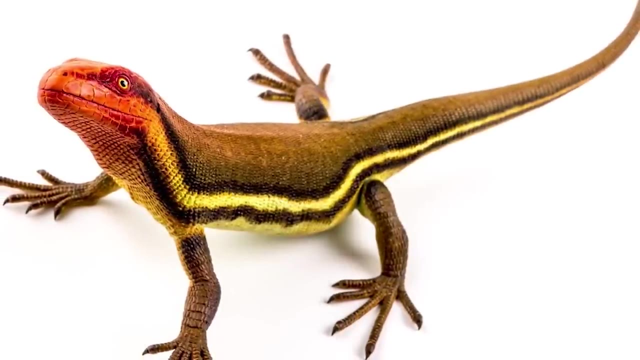 Joggins for decades, at one point blasting apart a reef to expose 25 trees. Fifteen were occupied. One of his discoveries, Helonymous Yelly, would later come to be recognized as the first reptile in the fossil record. He named it after Lyle Lyle's forest dweller. 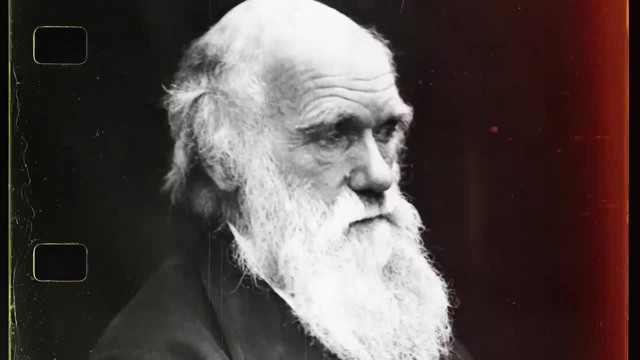 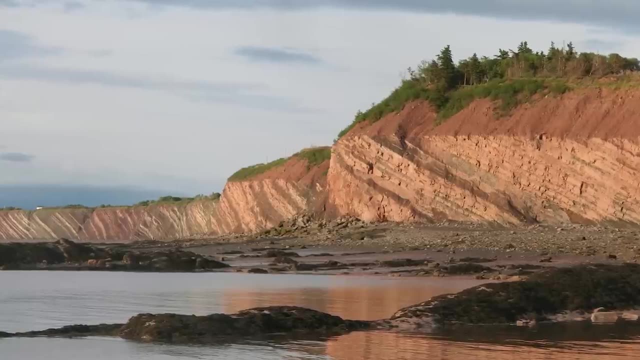 Charles Darwin found evidence for evolution in the Joggins' discoveries. Lyle and Dawson, on the other hand, found the opposite. Lyle's picture of gradual change over time had inspired Darwin to develop his theory of evolution. Lyle was unimpressed. 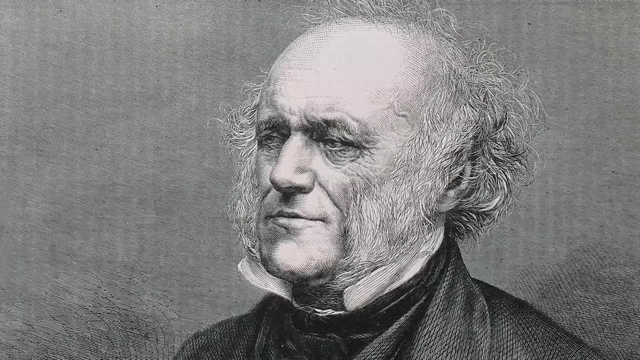 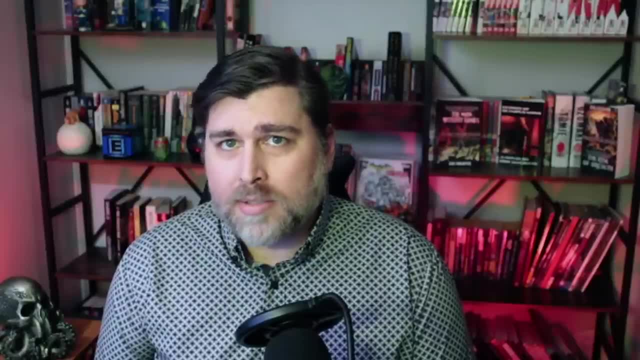 He thought evolution was able to appear temporarily credible because of how incomplete the fossil record was. Eventually, he was sure they would find evidence of higher lifeforms far back in the past. When the first hollow-tree tetrapod was found, Lyle took it as a win for gradualism and a blow to evolution. 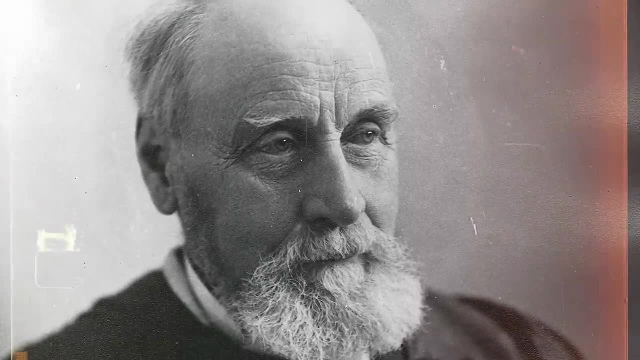 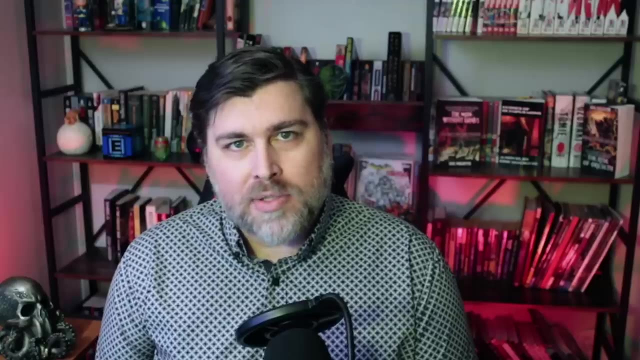 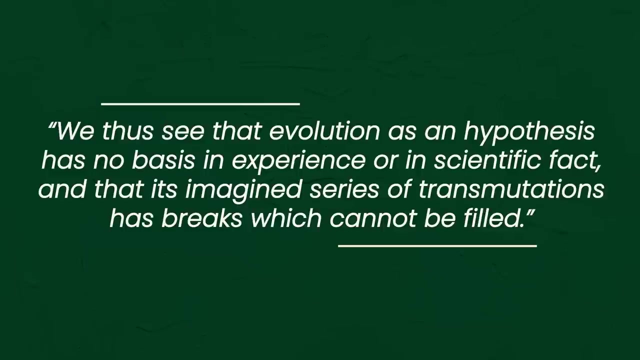 Dawson believed evolution contradicted his own observations at Joggins. He knew that some fossils were present and unchanged across millions of years. Nowhere in evidence was this slow, gradual shifting of form, He wrote. We thus see that evolution as a hypothesis has no basis in experience or in scientific fact. 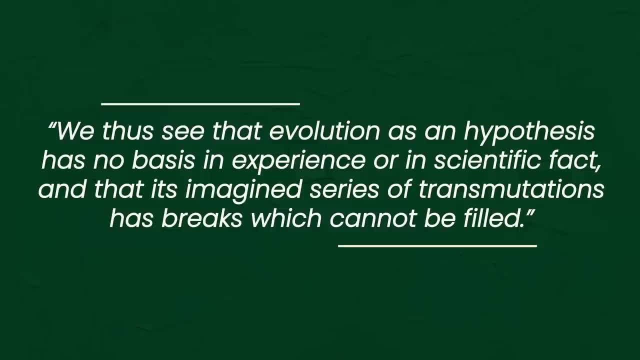 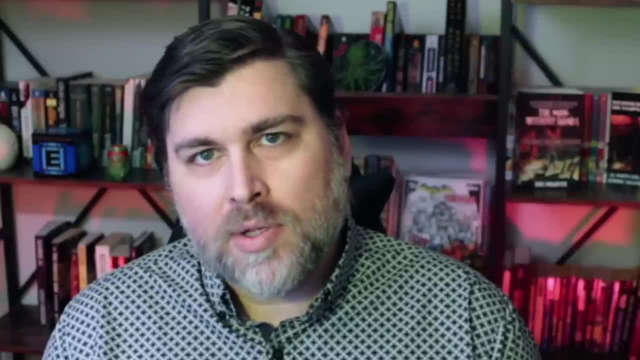 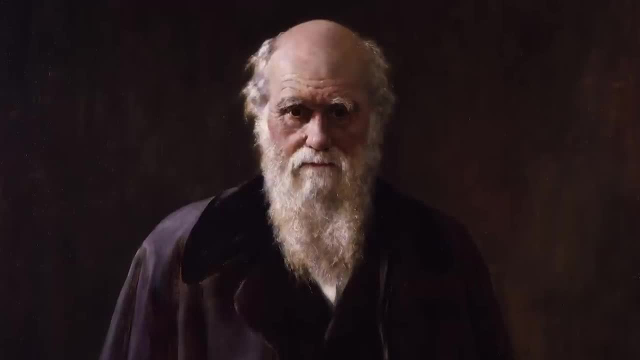 and that its imagined series of transmutations has breaks which cannot be filled. Dawson said Dawson's observation was true, even if his conclusion was not. We now consider that evolution can happen in short bursts with long stagnations. Darwin had anticipated objections on the grounds of insufficient fossil evidence. 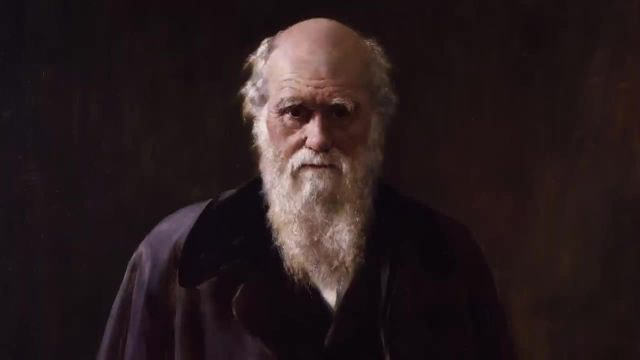 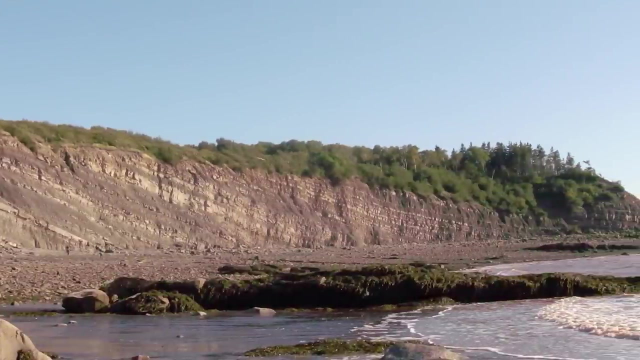 and on the origin of species. he used Joggins as an example against these objections. Joggins was put forward as the most complete site of its kind, Because we can see how wonderfully complete it is. we can also see how much is missing. Many forests were preserved, but most 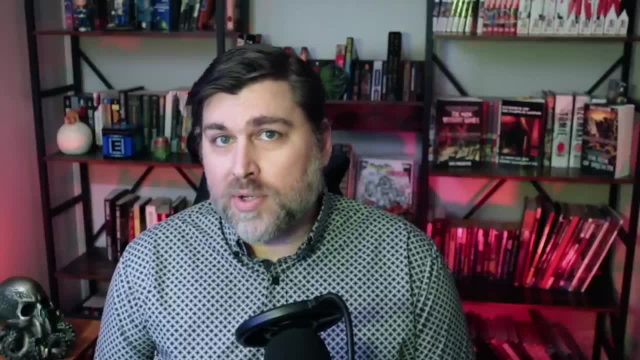 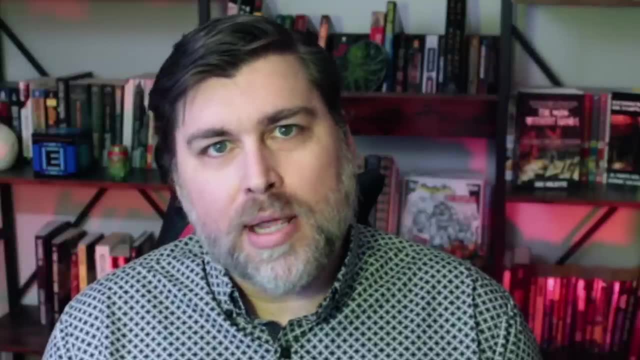 were not, During the times between those forests were still living. Most of what lives will never be preserved as a fossil. Finding fossils that unquestionably show evolution is nigh on impossible and cannot be taken as a requirement to accept the theory. 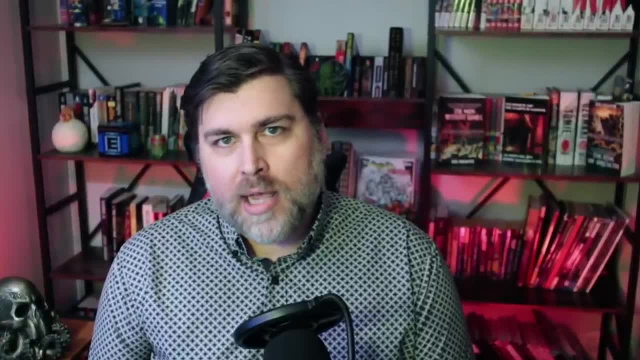 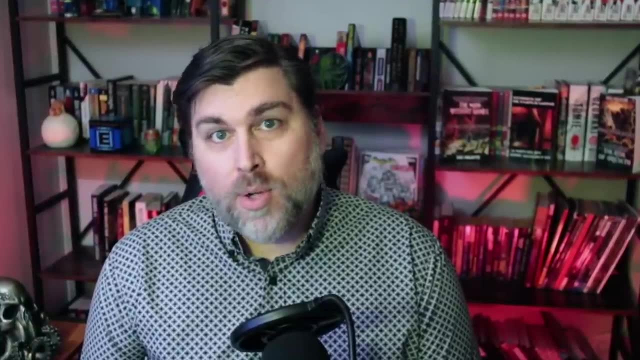 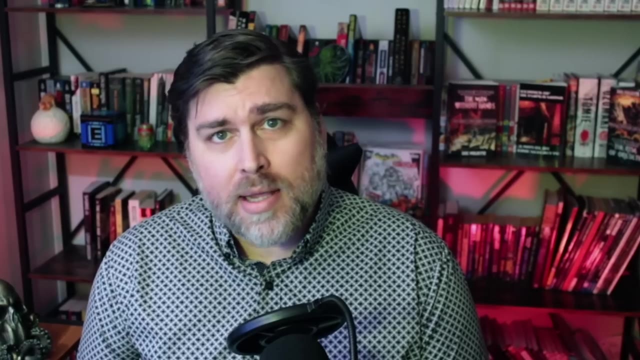 It is easy to take knowledge for granted, But things we know today as facts were once discoveries and theories. Once you have an answer to something, the evidence seems to point there Before you have an answer. it points everywhere, anywhere and nowhere. It may point towards wrong answers as easily as right ones. 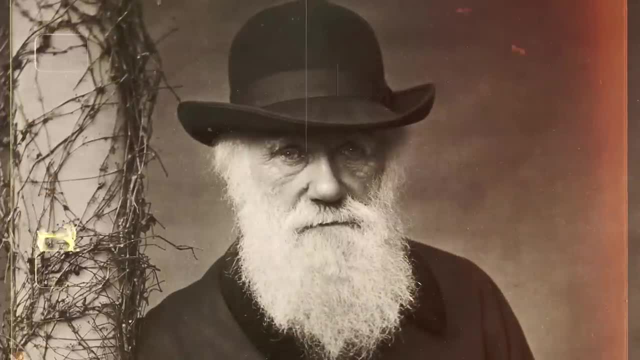 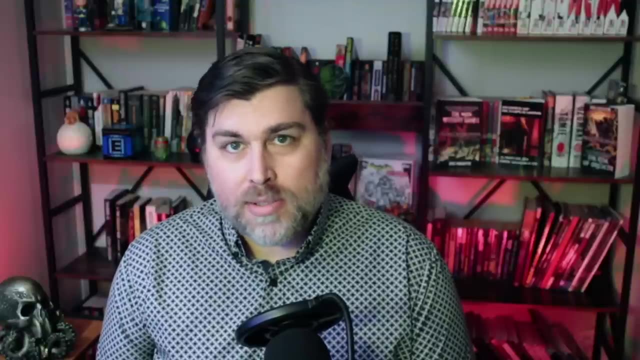 All of which is to say, Darwin did not know what coal was. He argued fervently about it with several esteemed scientists, including Lyell. In one letter to a friend, he furiously exclaimed: I suppose coal was rained down to puzzle mortals. 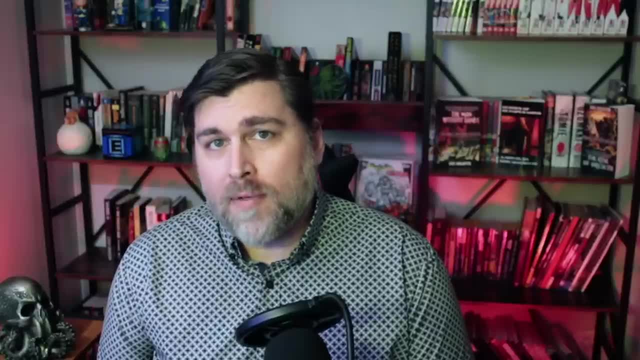 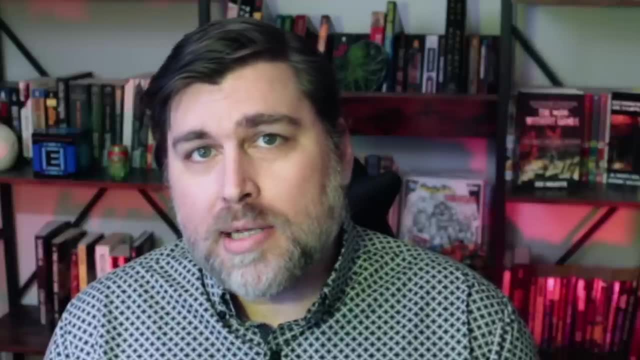 Darwin thought coal beds came from carpets of ancient marine plant life on the sea floor. Lyell and Dawson thought coal formed on land. That idea was the one that first drew Lyell to Joggins in 1842 after reading a geological description by a Nova Scotian coal mine manager. 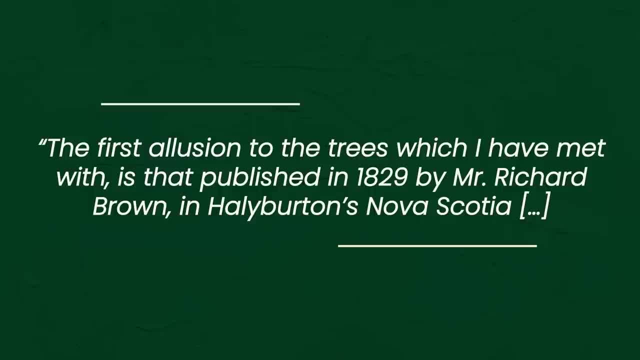 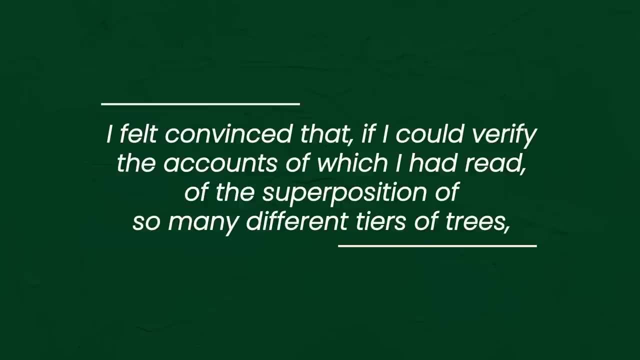 Lyell wrote. The first allusion to the trees which I have met with is that published in 1829 by Mr Richard Brown In Halliburton's, Nova Scotia. I felt convinced that if I could verify the accounts of which I had read of the superposition, 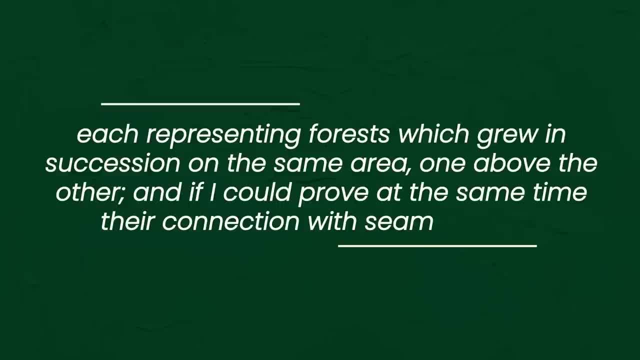 of so many different tiers of trees, each representing forests which grew in succession on the same area, one above the other. and if I could prove, at the same time, their connection with seams of coal, it would go farther than any facts yet recorded to confirm the theory that coal 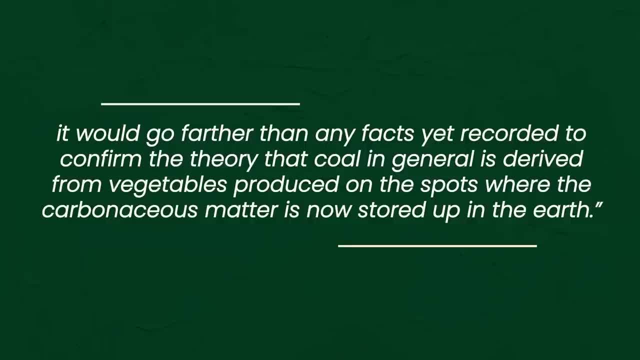 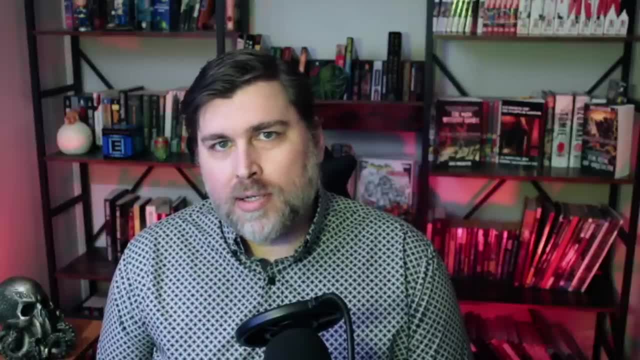 in general is derived from vegetables produced on the spots where the carbonaceous matter is now stored up in the earth, As it happened. he was right about coal and he was right that Joggins proved it, at least to Darwin's satisfaction. Calder calls the coal age. 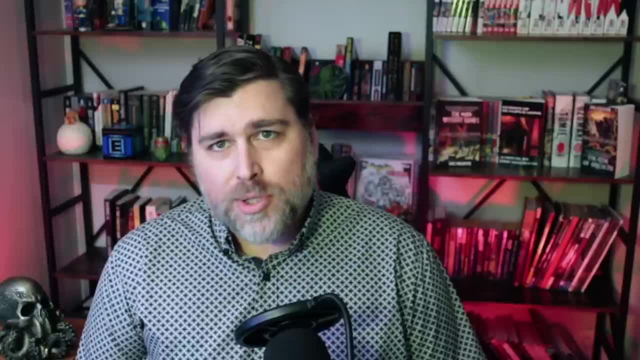 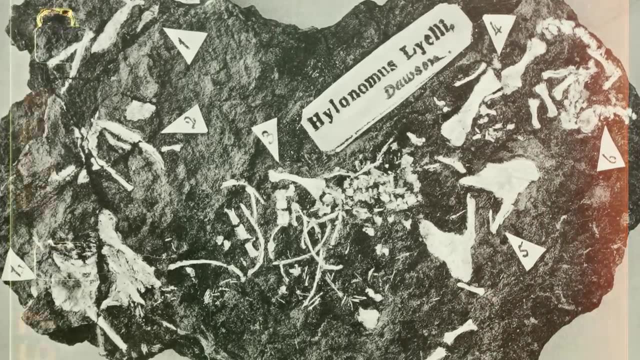 Act I of a two-act play. When Mr Brown wrote the description that drew Lyell to Joggins, it was in fact an early scene in the second act. The fossils at Joggins were found because of the search for coal, because of miners scuttling past ancient tetrapods in the dark. They were there for. 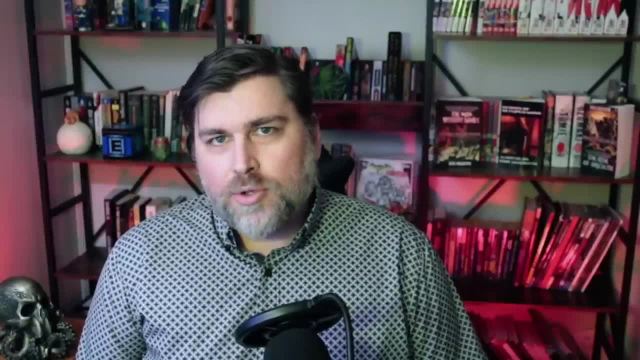 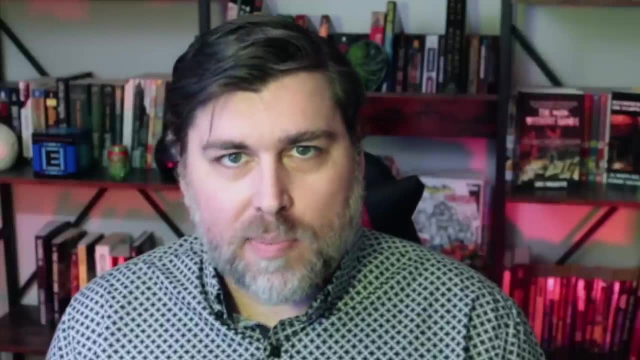 the industrial revolution there to keep the fires burning there to reshape the fate of the world by the simple action of making a livelihood. Now we are well into the second act of the play. The carbon that was long ago stored in the earth by carboniferous forests is being released. 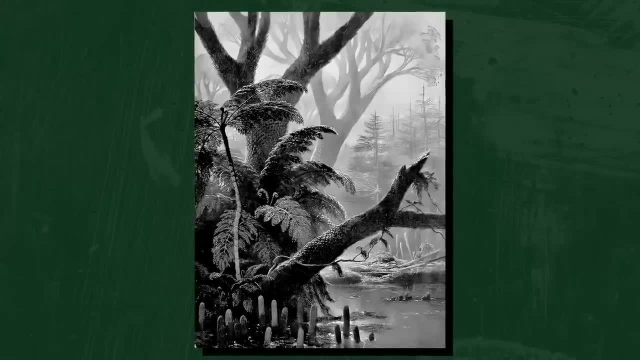 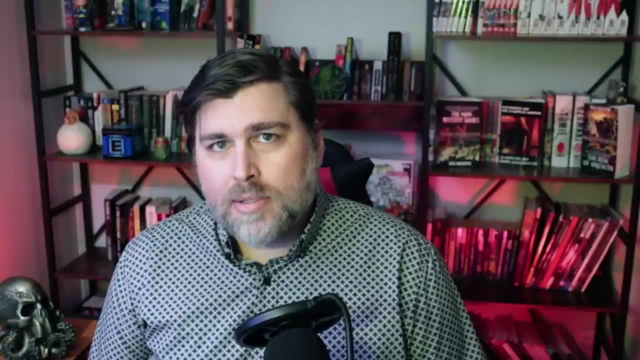 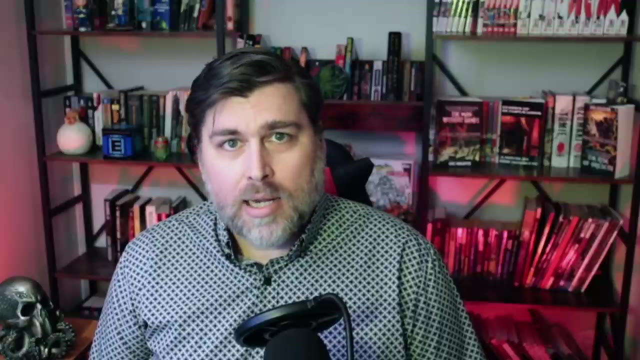 changing the balance of oxygen and carbon dioxide in the atmosphere. The greenhouse blanket is going back on the earth. Lyell said the present is key to the past. The past, in turn, may be the key to the present. By understanding the history of the earth, we change our understanding of current reality. 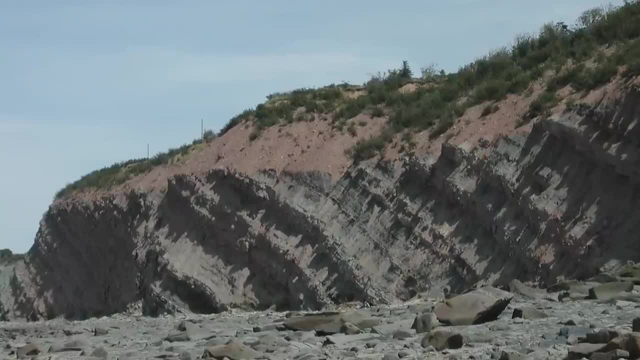 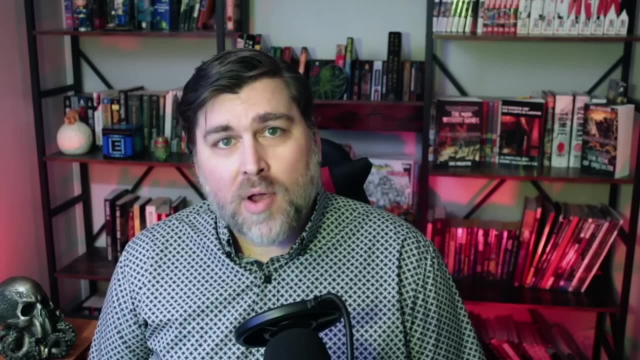 and can act upon that understanding. At Joggins we see a story of lifeforms profoundly changing the earth's atmosphere, altering the course of millennia. We see the immense consequences of carbon and oxygen. Calder urges us to read it as a warning. 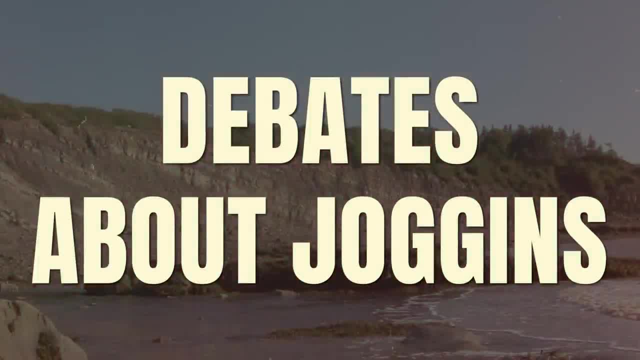 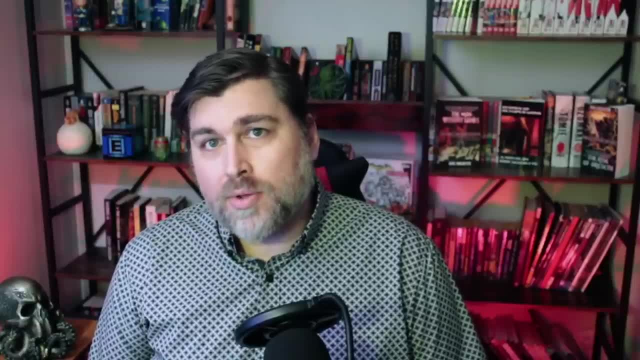 The top three episodes of Joggins are a series ofTo be continued. The Joggins site has played a role in debates of significance to humanity: Debates about the age of the earth, the nature of geological and biological change over time, the relationship. 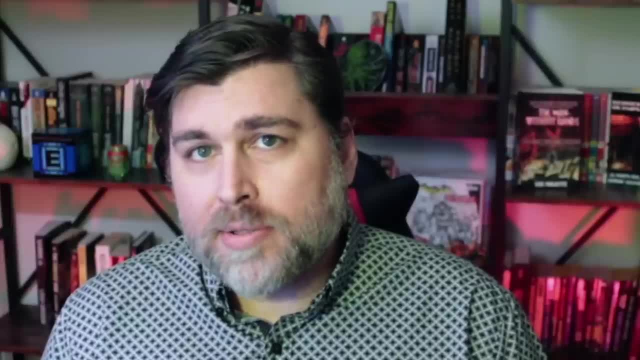 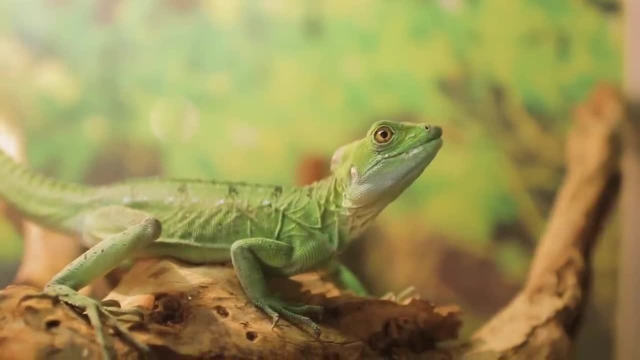 between the past and the present. There are a few smaller debates to bring up concerning Hellonymus, was it a reptile? Modern reptiles are scaly. They have some common features of the skull and vertebrae. They reproduce internally and their embryos develop in fluid. 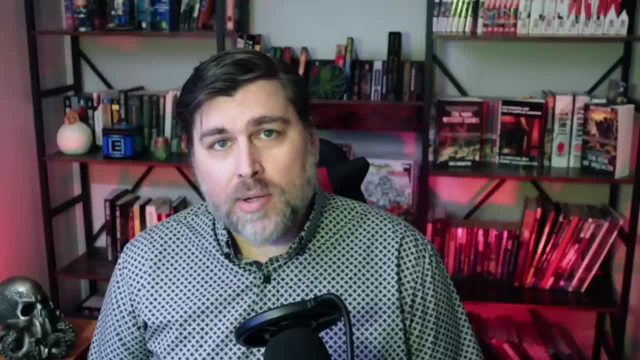 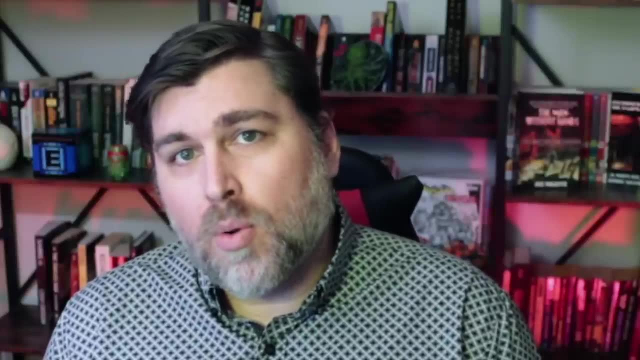 filled amniotic sacs. at the time of helonymous, early reptiles and amphibians were still distinguishing themselves. the reptile was learning to take the sea with it, its skin becoming more waterproof. the hard-shelled egg, a portable sea you can lay anywhere- is usually cast as the 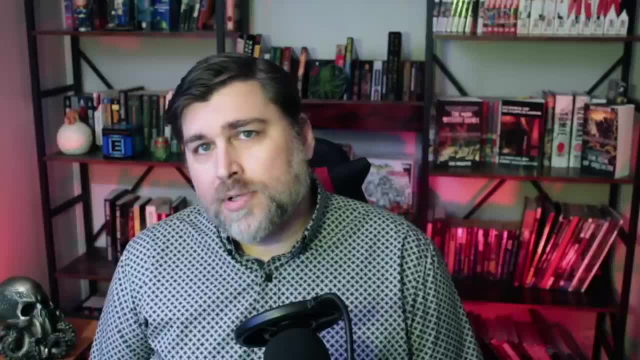 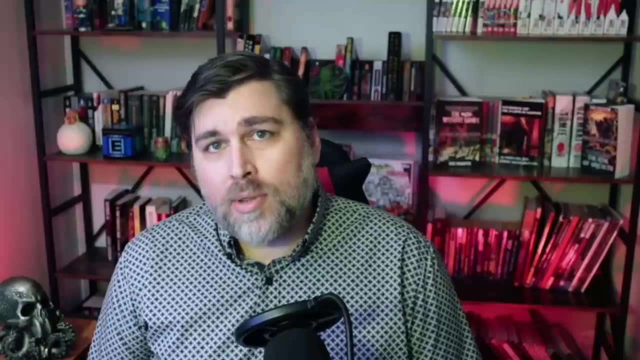 definitive step toward reptilian independence. no fossil eggs have ever been found at joggins. a recent study has called the essentiality of the egg into doubt, suggesting that early reptiles might have been able to bear life young. the definition of reptile has changed several times. 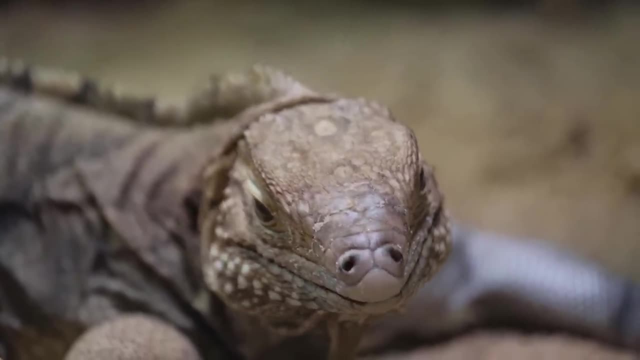 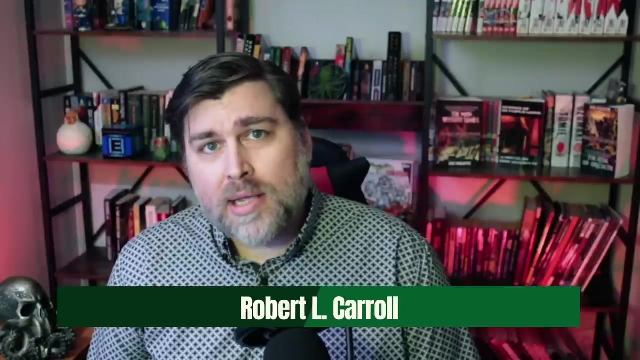 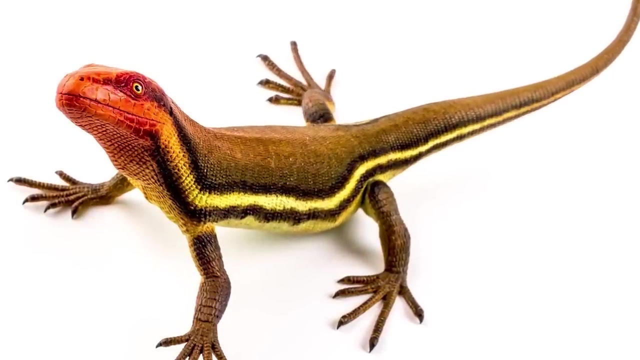 what we really want to know by is it a reptile is? where does it fit on the tree of life? how are we related to each other? a hundred years after helonimus was found, paleontologist robert carroll officially granted its status of the reptile class: it may be the earliest member of one of the three. 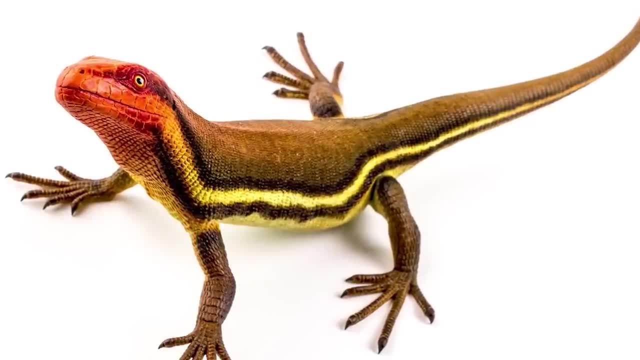 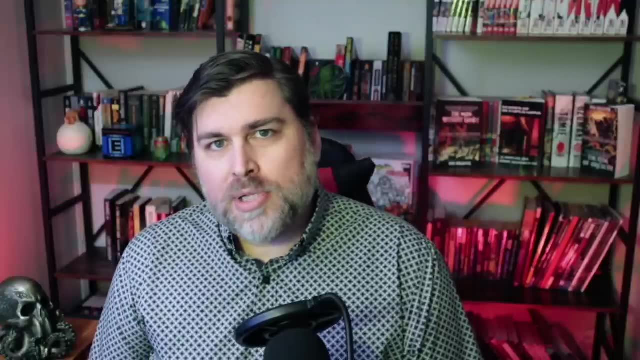 main branches of reptile, but those branches are still hotly contested. the second debate about helonymous is: what was it about helonimus that made it possible for the reptiles to be able to survive in the wild, and what was it doing in the lycopside when lyle and dawson first presented? 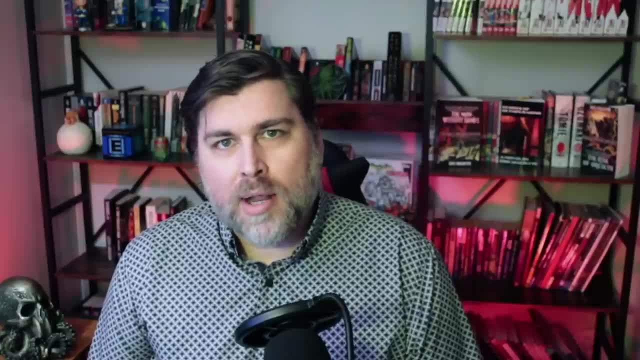 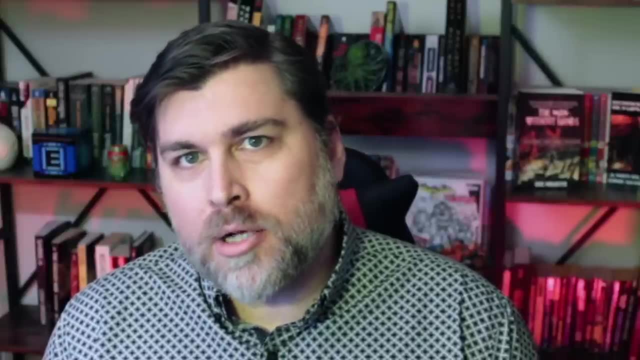 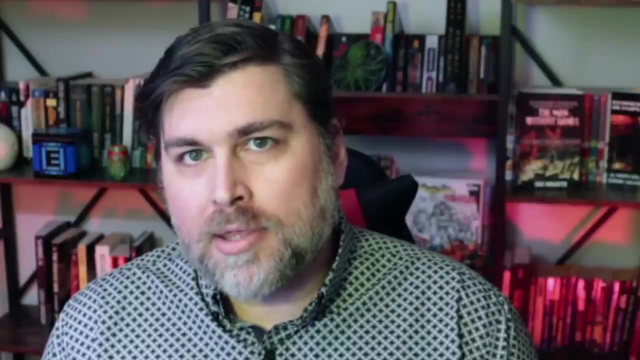 their discovery of the hollow tree creatures. they offered three theories about how the creatures got into the trees. one: they used hollow lycopsids as dens. two: they were washed in by flood waters. three: they fell into pits created by the hollow buried trees and were trapped there to death. dawson. 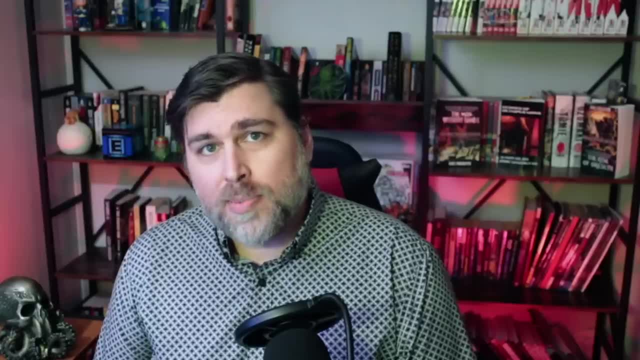 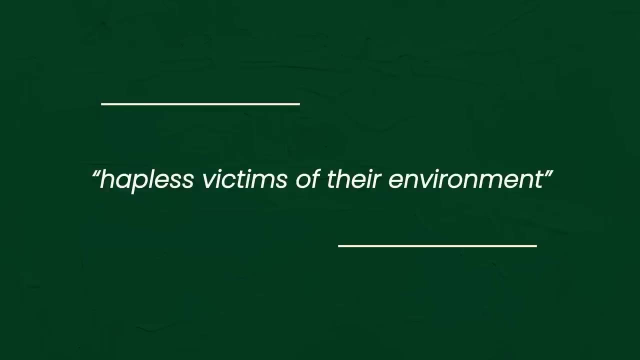 favored the pitfall theory. calder calls the inclination towards pitfall theory a human-centric, victorian view of nature, casting animals as half-baked trees and the other half-baked trees hapless victims of their environment. he argues for dents. the creatures are found in the base of the. 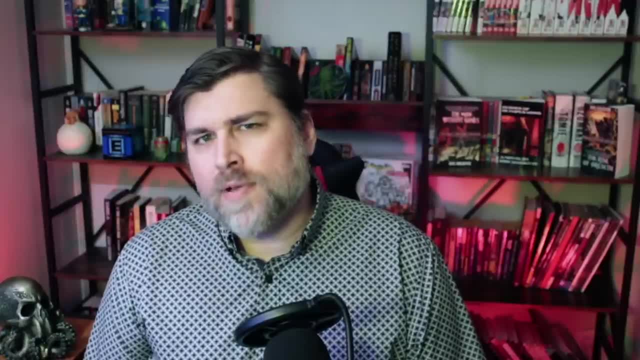 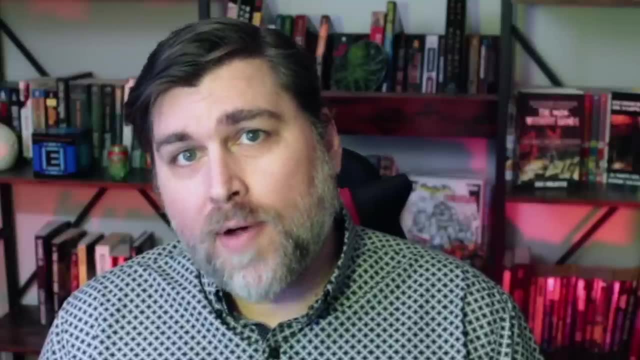 trees. beneath the sediment that washed in later they are usually found with fossil feces, so they were alive inside the trees for some time. they are always found with fossil charcoal, so fire was always involved. the fire scars on the lycopsids could have made for points of entry in the 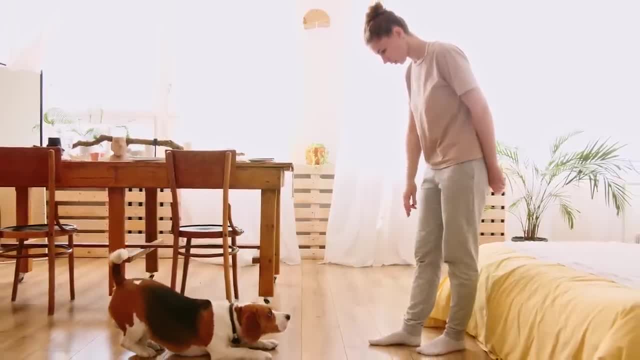 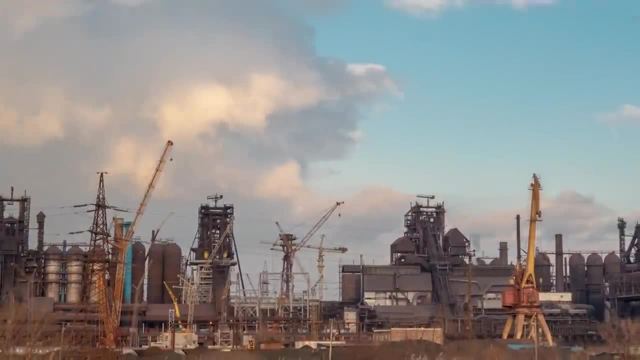 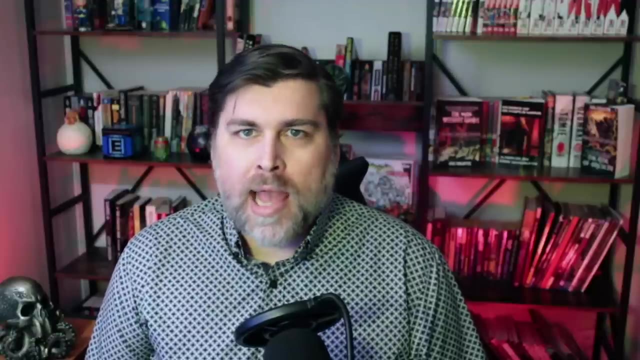 victorian view of nature. humans stand alone among the animals. humans act with reason. humans bring the coal fires of the industrial revolution, the fires of progress, the fires of enlightenment and advancement. it is for humans to read and interpret the book of time. we are the active agents on the